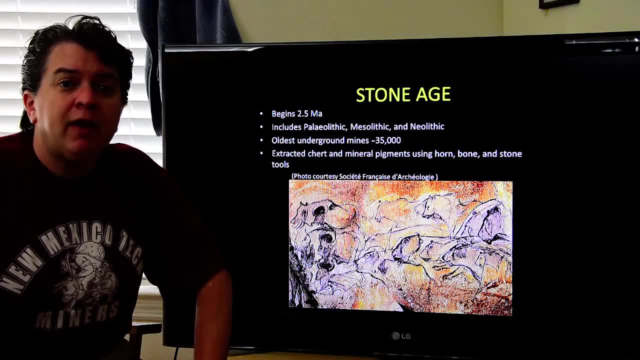 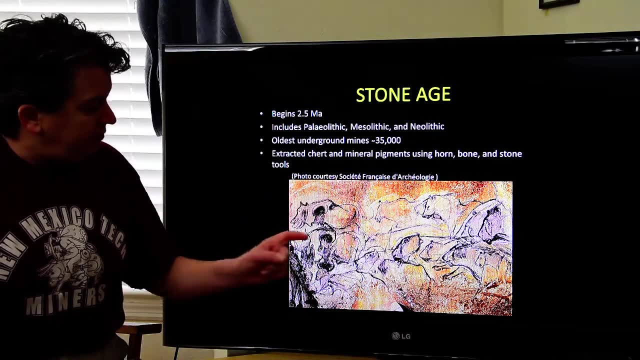 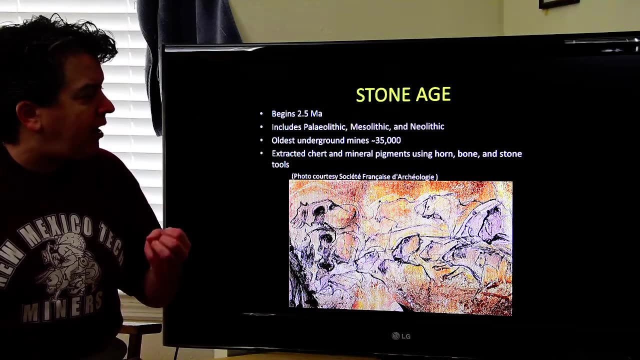 chert or flint, which would be made into things like arrowheads and spear points, but they also extracted mineral pigments so they could make artwork like this. And how did they get that stuff out of the ground? They used horn, bone and stone tools, And this limited them to. 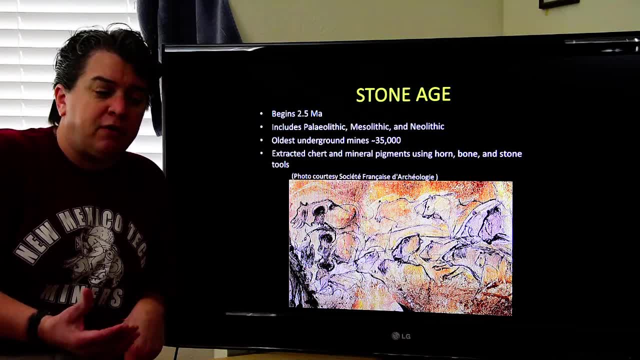 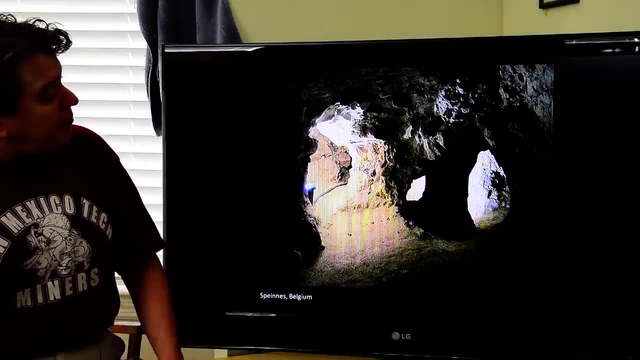 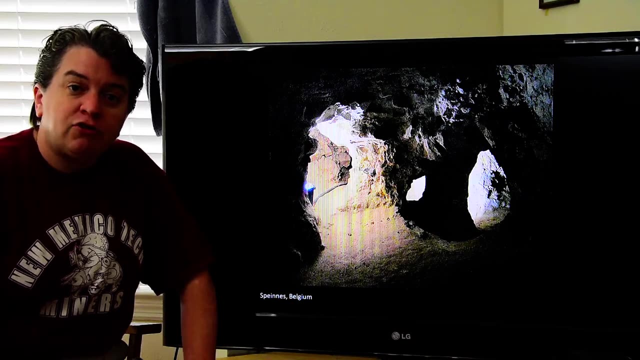 extracting materials out of softer rocks, because those tools are not going to be very effective against really, really hard rocks. This is a Stone Age mine in Belgium. that's from a well-known an underground mine where they would extract chert. Now, following the Stone Age, we enter. 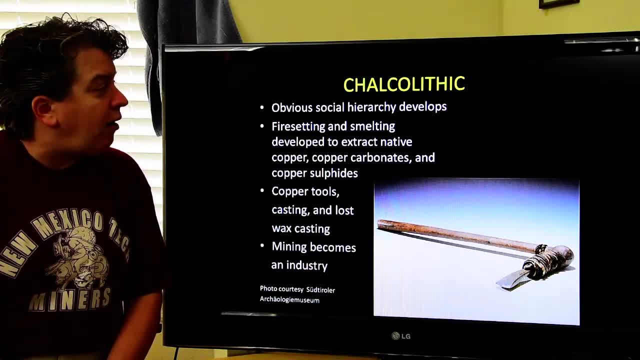 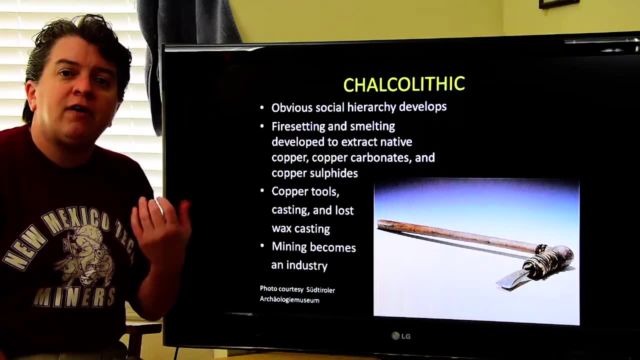 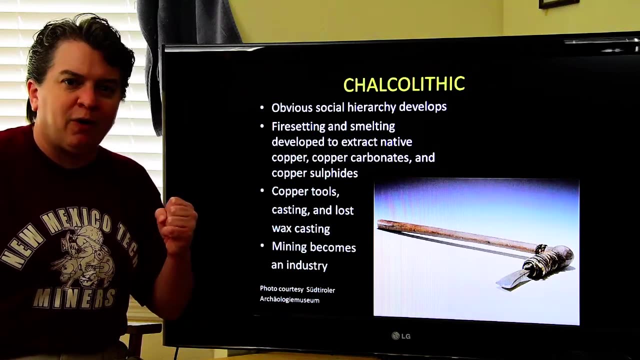 a time period called the Chalcolithic. It's also sometimes called the Copper Age, And in the Chalcolithic we start seeing a very obvious social hierarchy, Because when you excavate Chalcolithic sites, there's definitely people who are wealthier and definitely people. 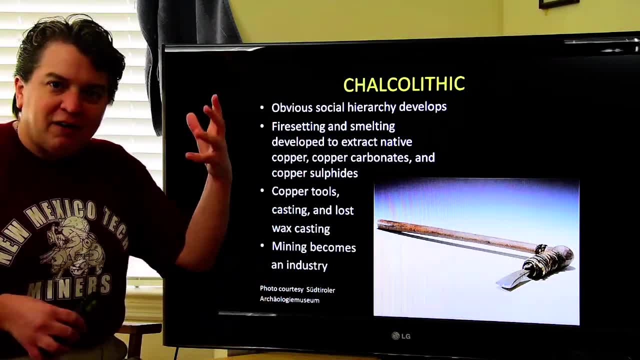 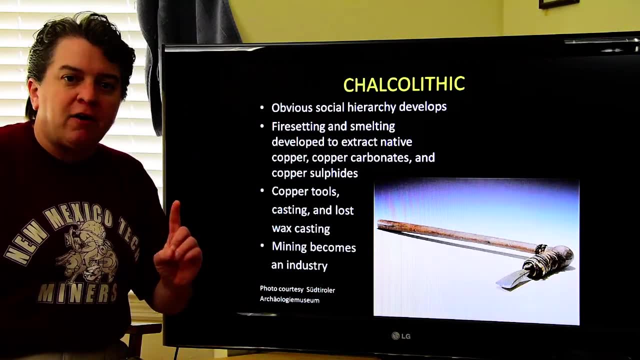 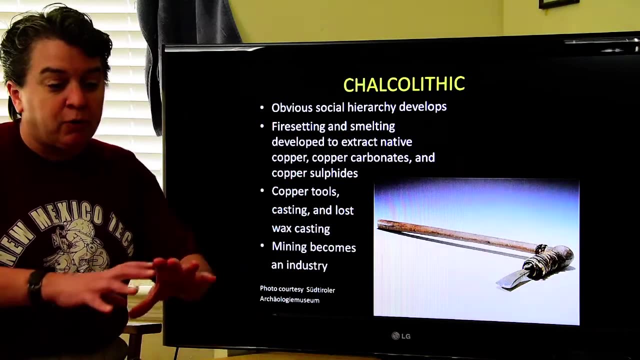 who are not so wealthy. So we start seeing kind of this hierarchy. A big development for the Chalcolithic was the development of fire setting and the development of smelting. Now fire setting is where you would build a really, really big fire up against some. 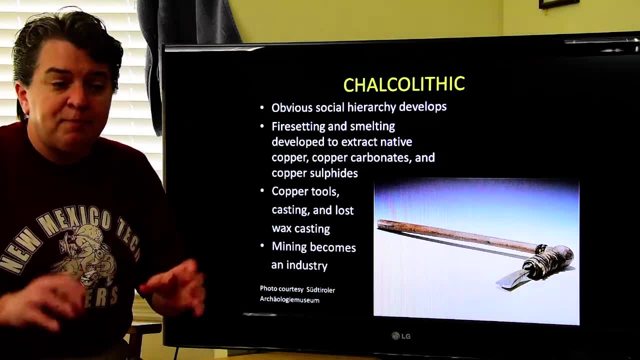 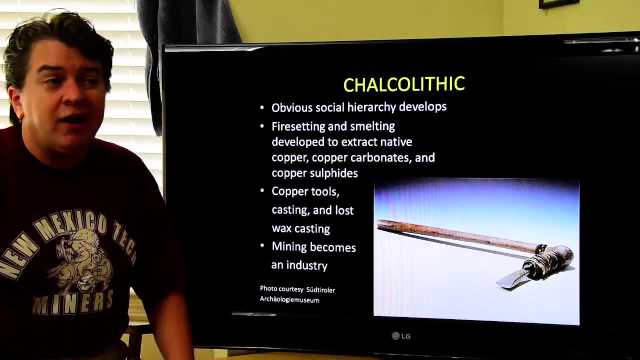 hard rocks. get those rocks heated, and what this would do is it would soften them, It would break them down, make it easier to break them apart. Sometimes you'd even heat them up and then dump really cold water on them, And what this? 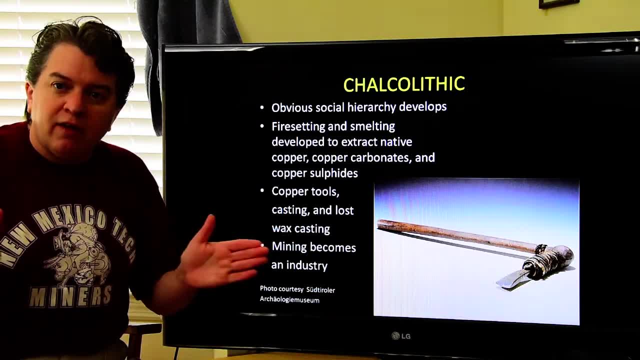 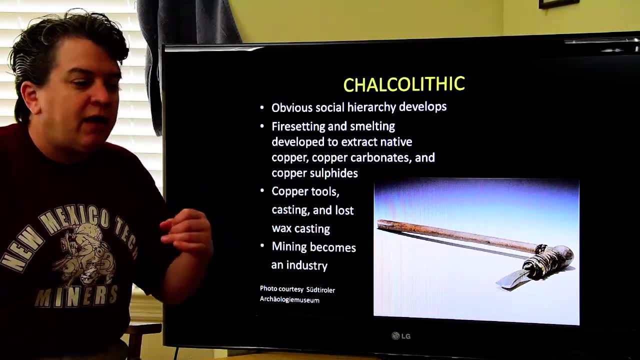 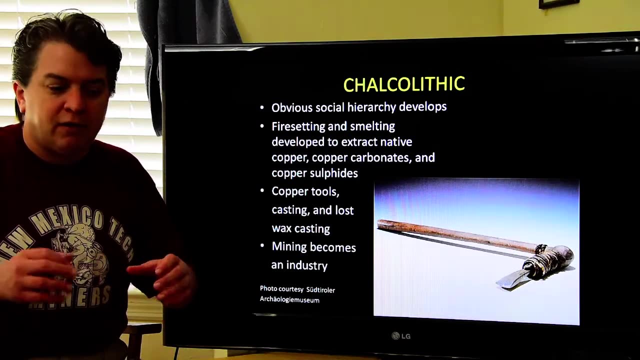 would do the sudden. when things get hot, they expand, and when they cool down, suddenly they contract, and that could crack the rocks. And so now these people of the Chalcolithic are able to extract minerals out of harder rocks, because they figured out a way to break. 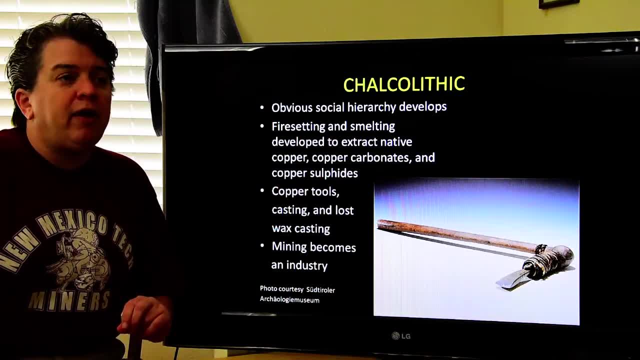 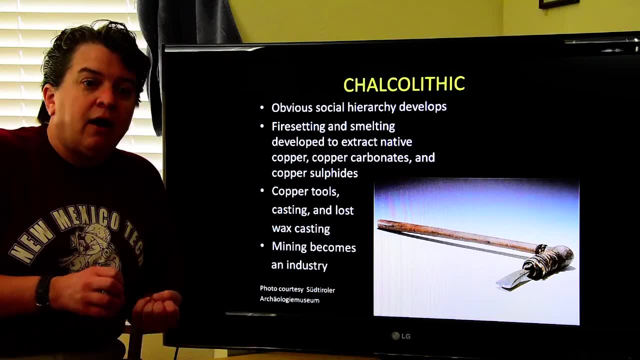 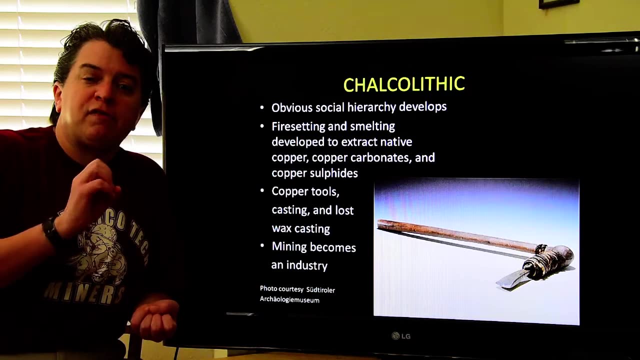 them down. Now, smelting is where You basically grind up a rock and you melt it, and when it gets melted, you get your- in this time period- copper, your metal, and then you get something else called slag, which. 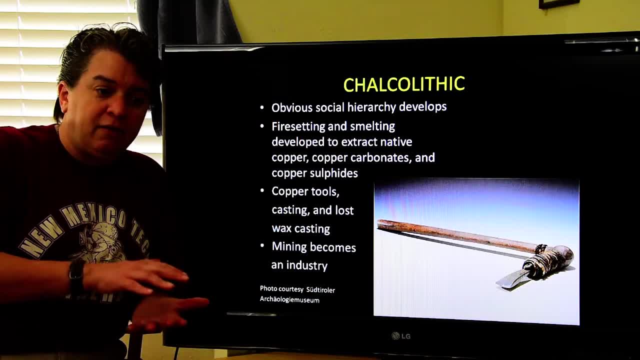 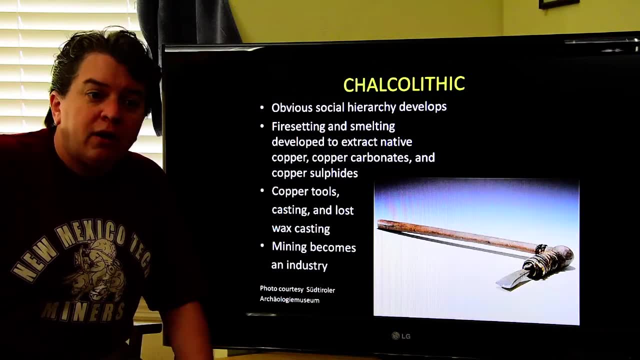 is the not so good stuff And the slag, basically, is less dense, floats to the top, you can pour off that stuff and then you're left with your nice pure copper. And so, since fire setting and smelting were developed, people are going to be able to. 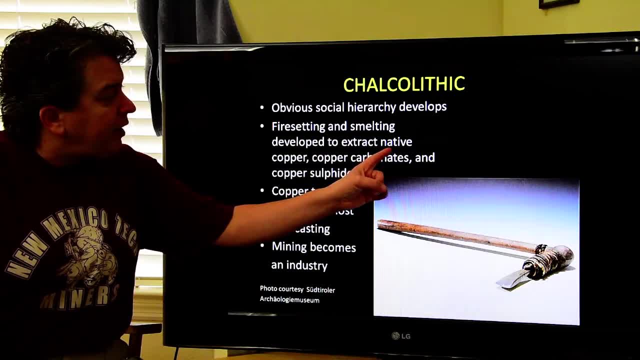 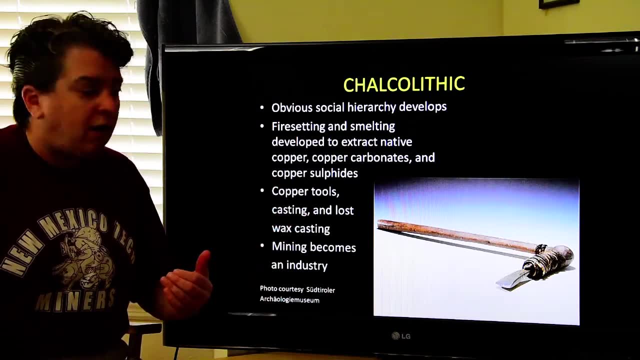 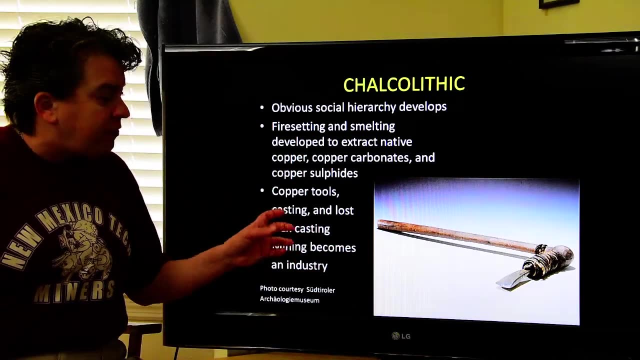 extract more minerals and they're going to now be going after native copper. that means pure copper. They're going to go after copper carbonates and copper sulfides to extract the copper and make tools out of them, like this axe. So at this time they make copper tools. they shape these tools or form them using casting. 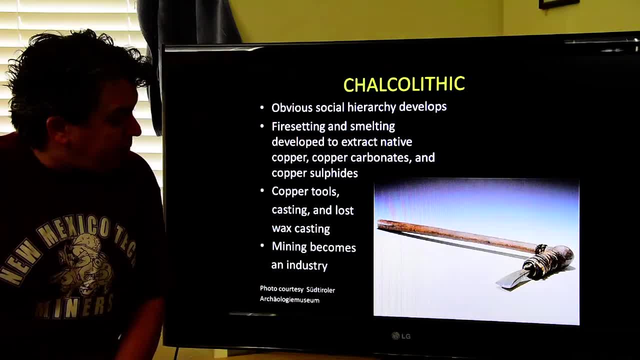 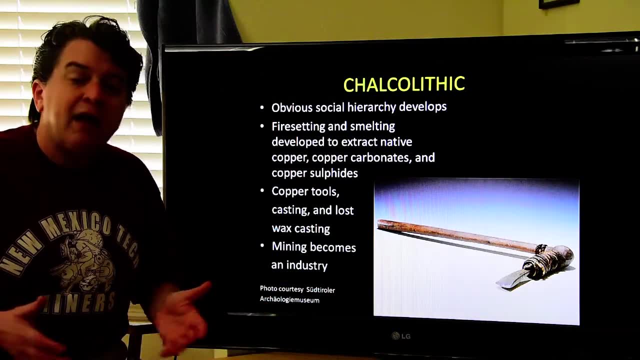 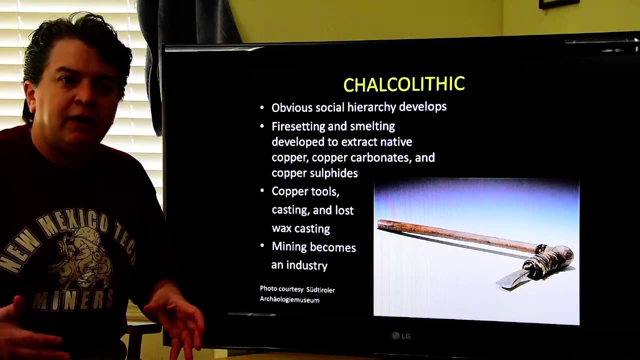 and lost wax casting, And at this point mining becomes an industry. Now, how do we know it's an industry? Well, these sites have been excavated, where we can see it wasn't just an individual person or a family doing this activity, but a number of people like 30, 40 or more people, all. 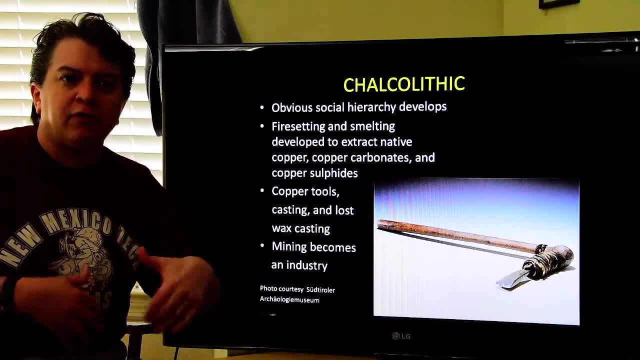 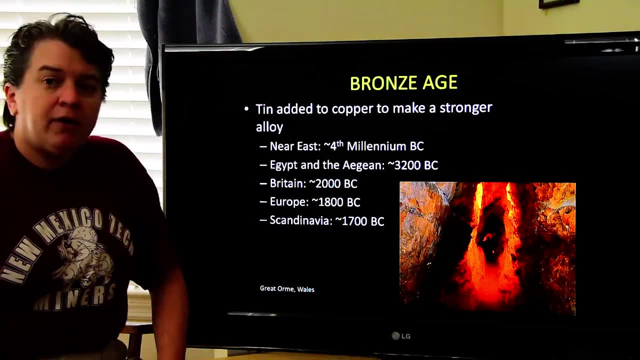 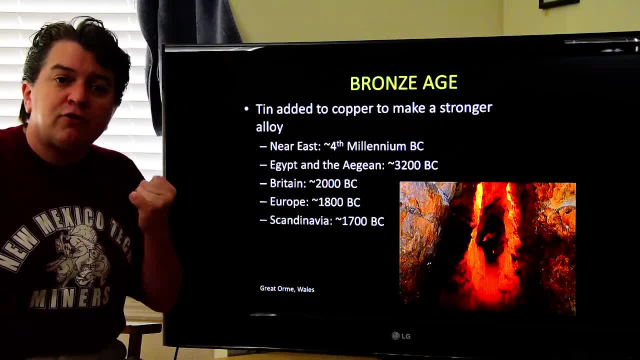 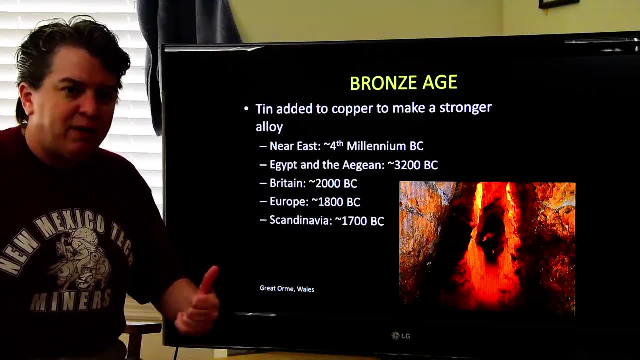 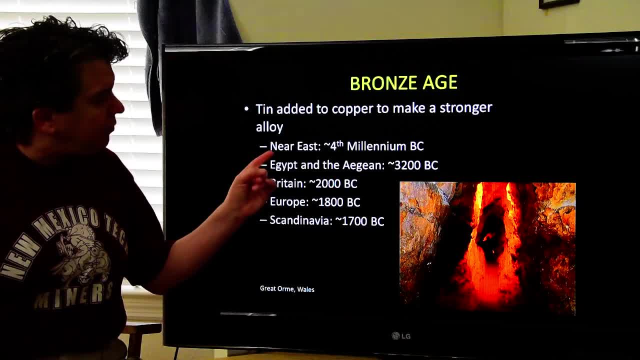 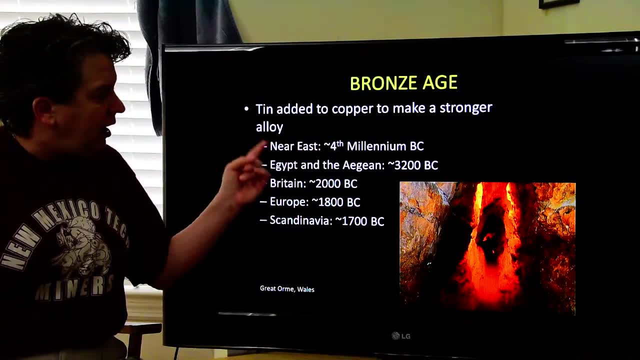 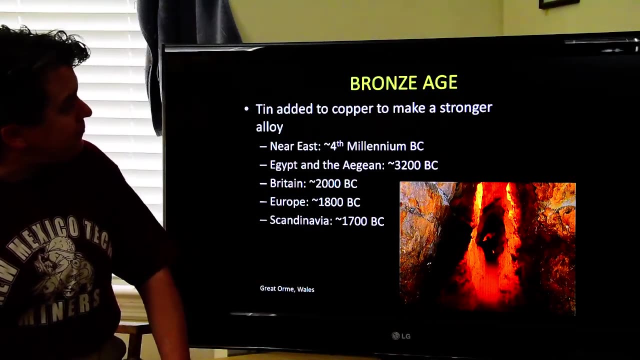 Now, as I said, these are technological developments, so we can see the Near East. in the fourth millennium BC we begin the Bronze Age And my people in Scandinavia they got it kind of late. Now, following the Bronze Age, we get the Iron Age and the Iron Age begins in the Near East. 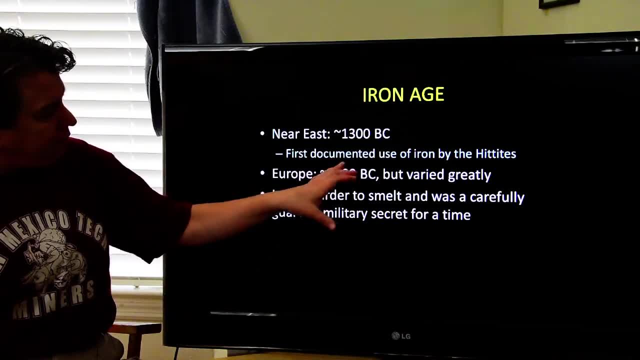 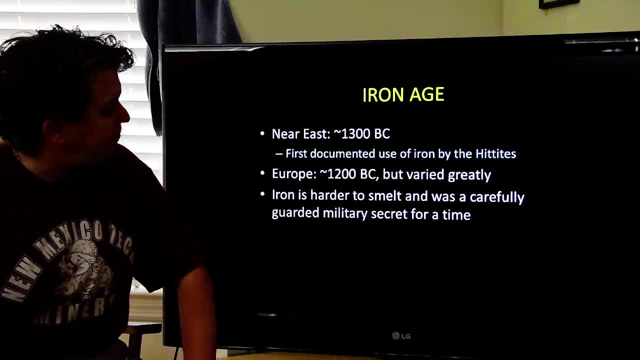 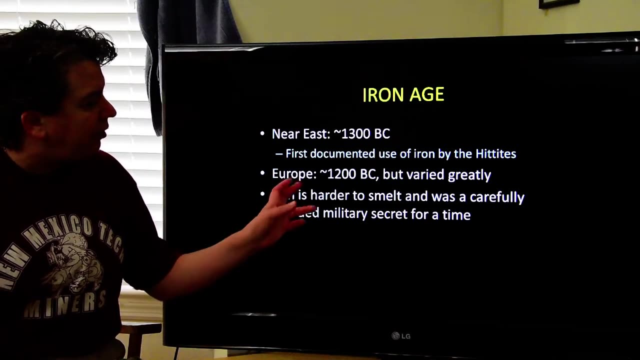 around 1300 BC. The first documented use was by a group called the Hittites and they lived in what would be modern day Turkey. and it arrives. the technology for smelting iron arrives in Europe by about 1200 BC, but the actual date varied greatly. 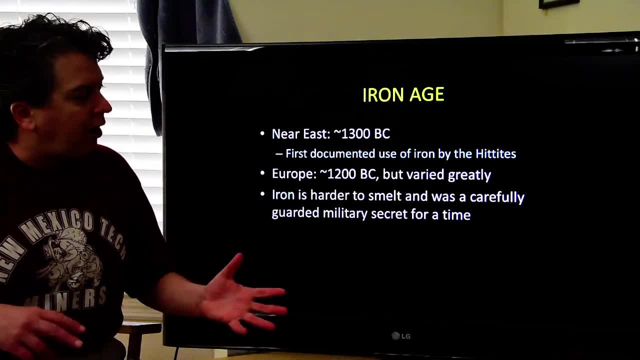 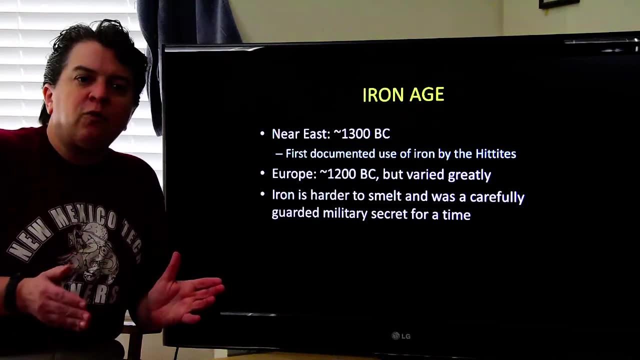 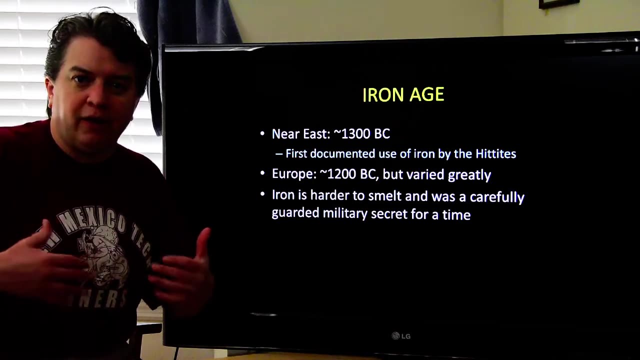 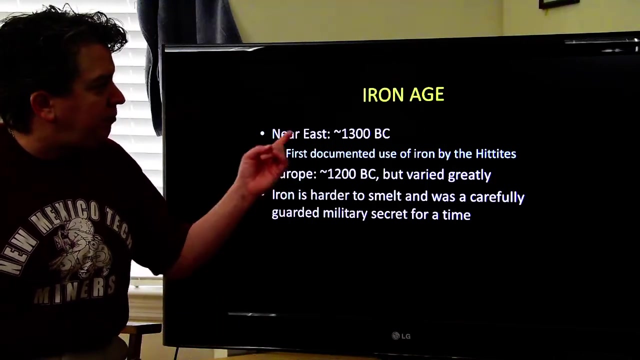 Iron is harder to smelt than other metals, and so for a while this was a carefully guarded military secret, because iron weapons were much stronger and much better, and he who would have the better, stronger weapons could rule the world right. So it was a carefully guarded secret, but, like all good secrets, pretty simple. 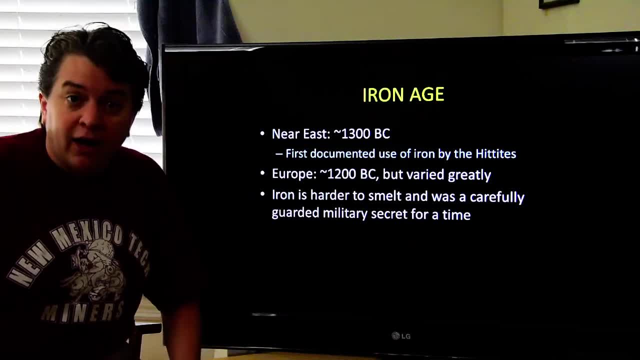 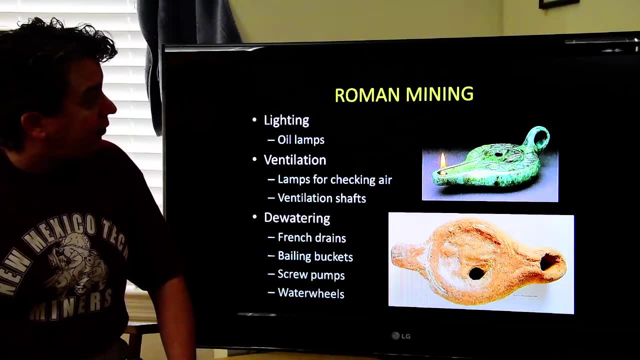 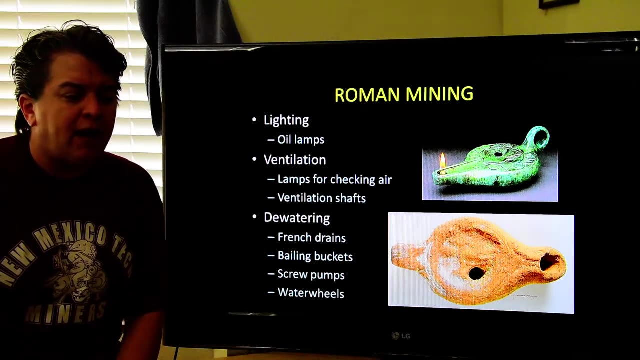 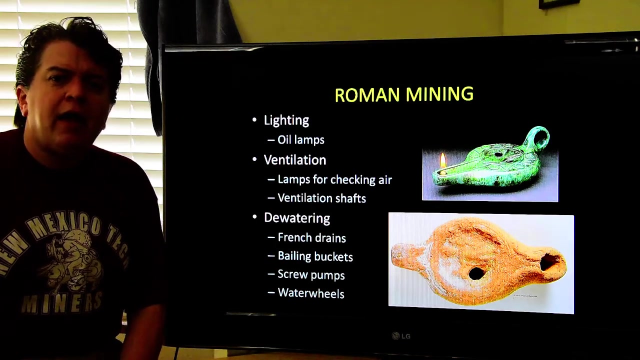 Prehistoric WikiLeaks or whatever it got out, and this use of iron ends up spreading throughout the Near East and Europe. Now, eventually, we get to the Roman time period and the Romans were absolutely amazing miners and engineers because they started getting deeper and deeper mines underground and when 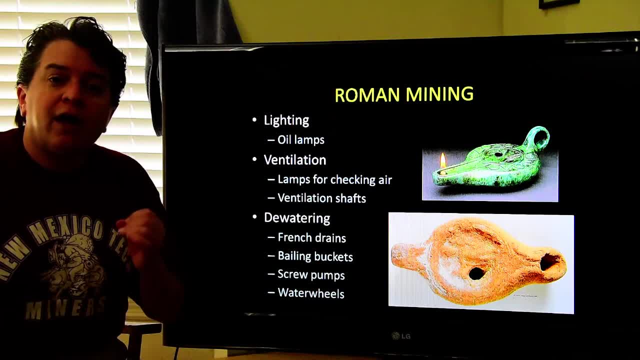 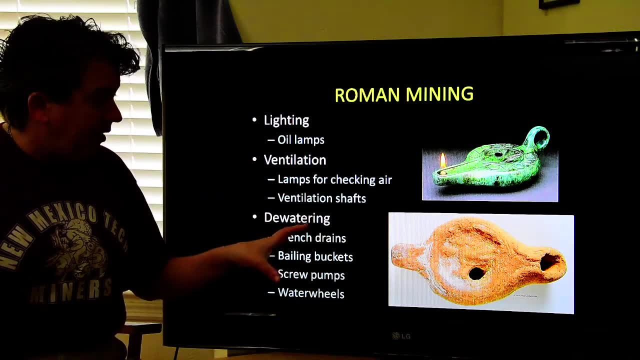 you start going this deep underground, you start having a few issues. You have to light things, you have to get air circulation going and groundwater is going to start seeping into that mine, so you have to get it out. Well, how did they solve these things? 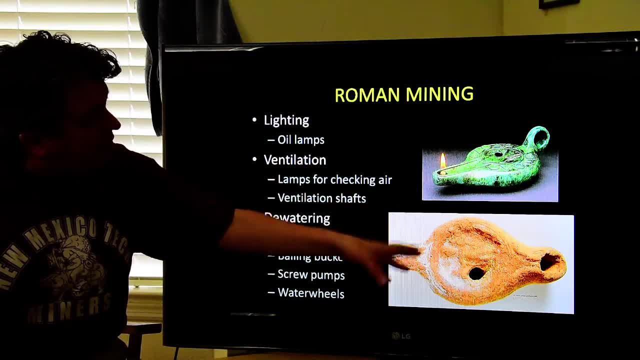 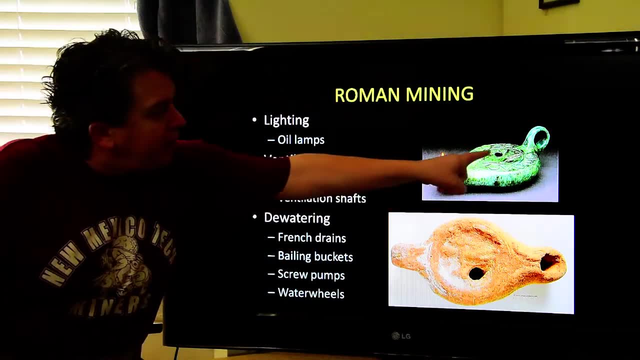 They lit the mines with oil lamps like this, and I put this picture in just because this shows an oil lamp in use. we have the wick there. you'd fill this with olive oil now. that would be like what you have in your house, because that's really nice. 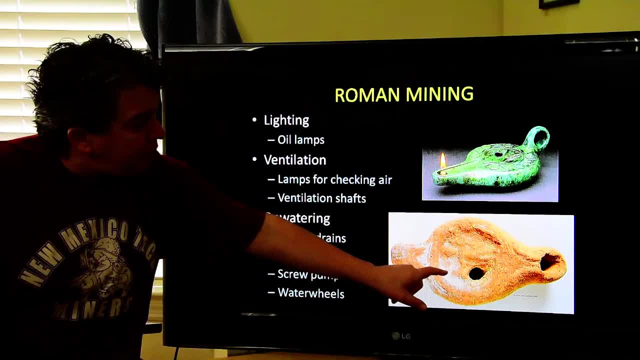 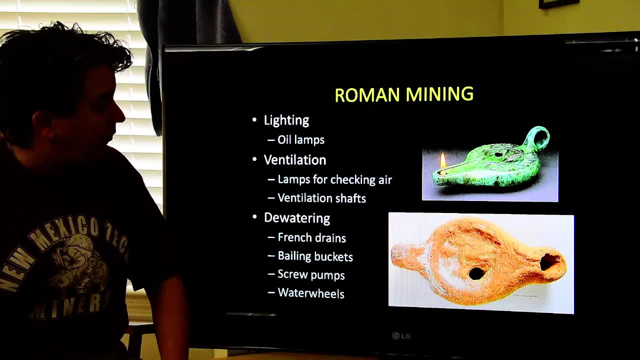 In the mine. they just have a very simple terracotta one like this, but it would work exactly the same way. You fill it up with olive oil. there'd be a wick there, and that's how you're going to light your way underground. 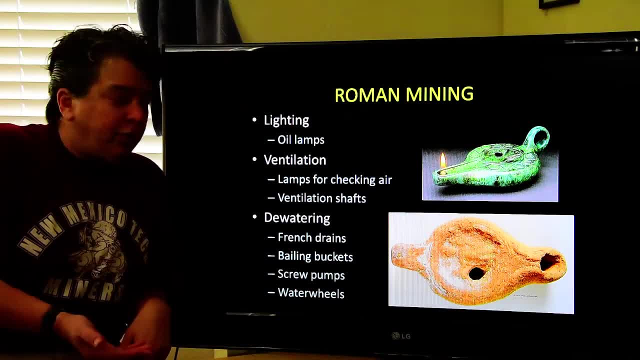 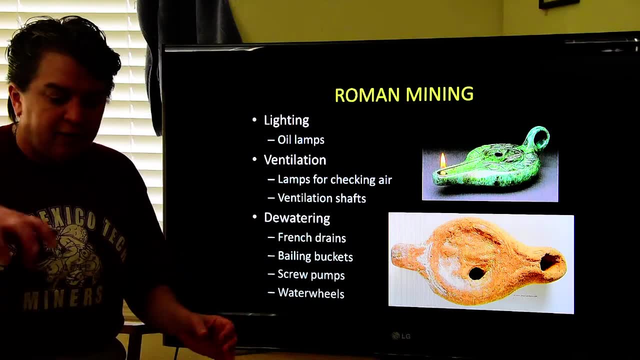 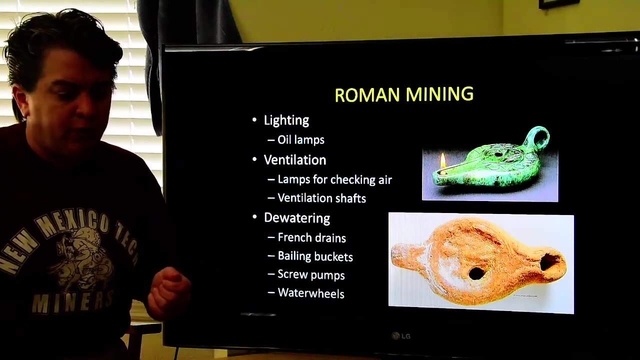 Now, like I said, when you get deeper underground you need to make sure there's air circulation, and the Romans would actually dig special shafts to get circulation going around the mine. They even have recorded that they would lower these lamps into a mine to make sure there's. 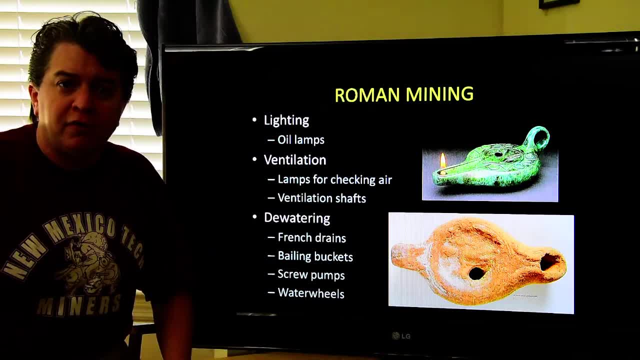 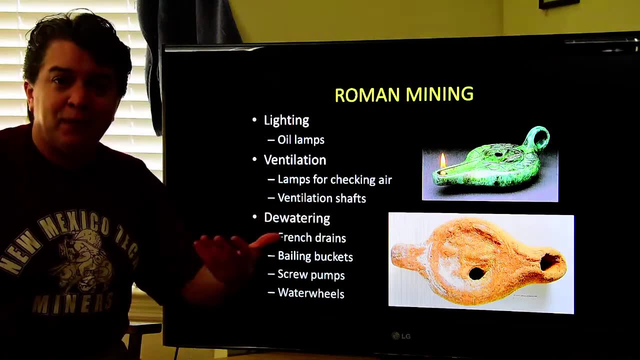 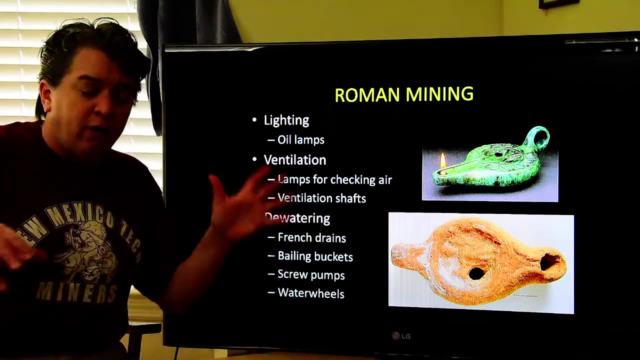 no, what we call dead air, air with no oxygen in it, Because while they might not have understood the fire triangle and what oxygen is, they knew both fire and people needed something that was the same If their ventilation shafts wouldn't work and get a good flow of fresh air in the mine. 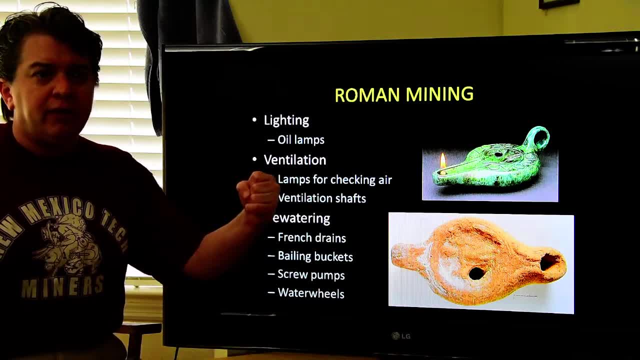 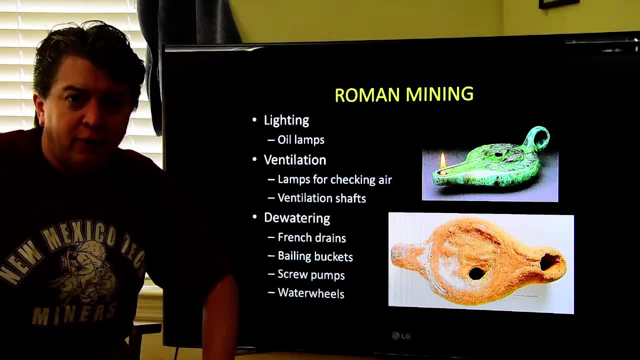 they actually had some poor dude who had like a big linen towel and he'd stand at the opening of the mine and wave the towel and force air into it. When I think that I don't like my job, I just think what it would be like to have that job. 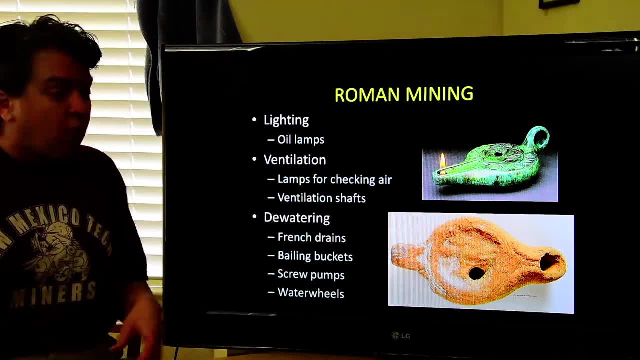 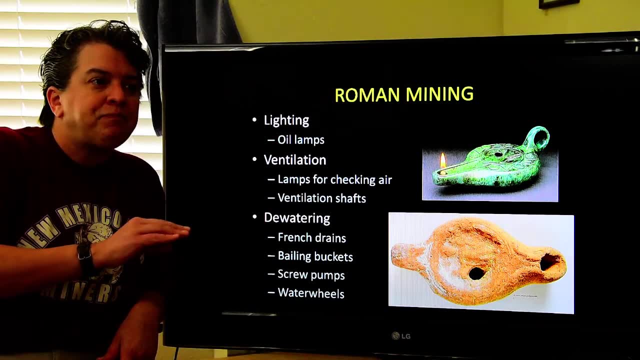 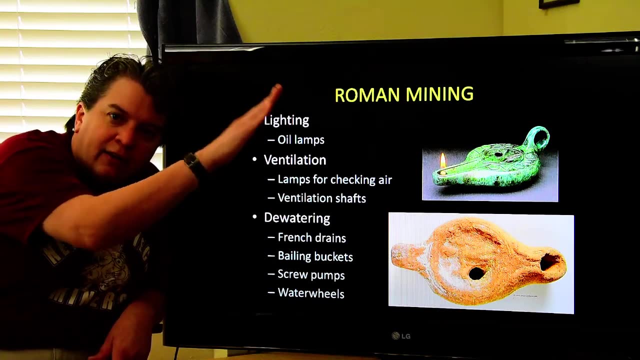 So anyway, that's their solution for ventilation. Now dewatering: they sometimes used French drains, which is basically where you just have. You just have your mine tunnel going into like a mountainside, But you incline it just slightly so water will flow out of it. 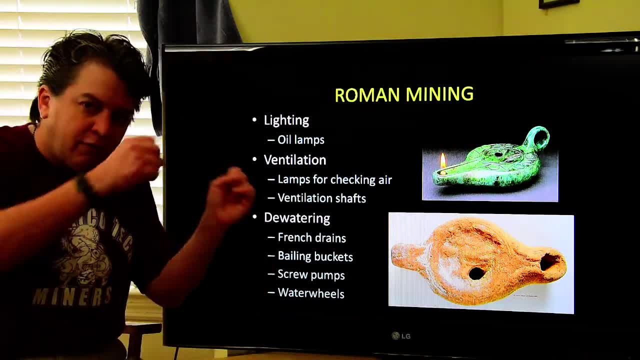 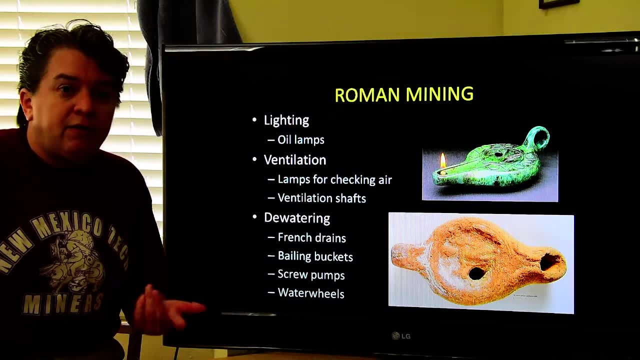 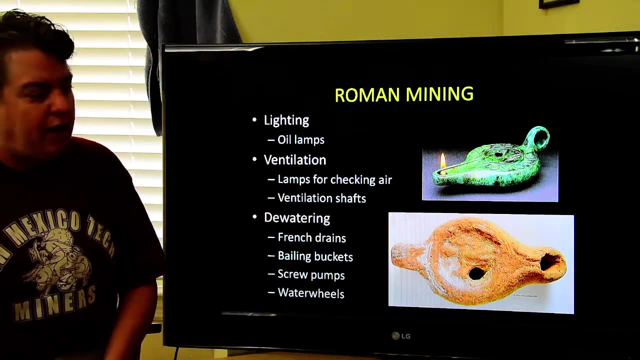 They used bailing buckets, where you just lower a bucket down and just constantly you know bail things out, Although they also had screw pumps- and that's a very early type of pump that, in fact, the ancient Greeks developed- and they would use water wheels. 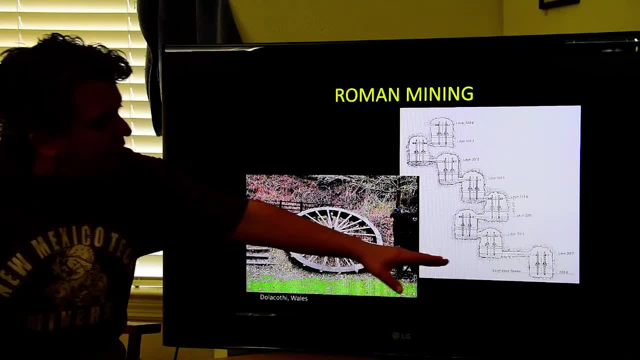 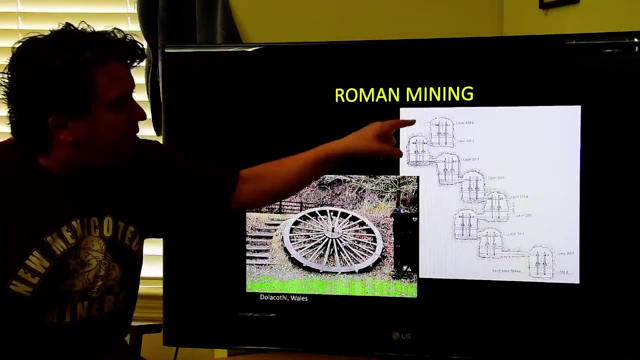 And this is quite ingenious. So underground, they would have a series of water wheels Here, this one would lift it up to this level, and that would lift it up to that level, and so on, And that could lift water hundreds of feet out of a mine. 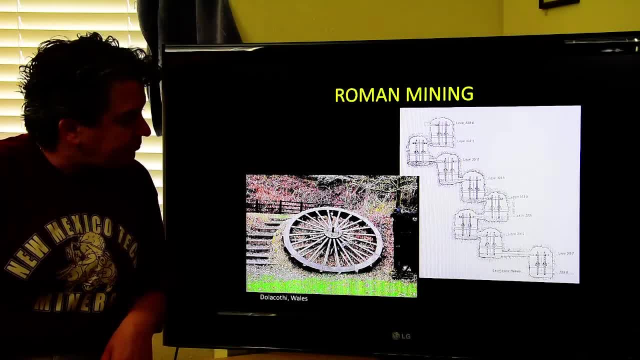 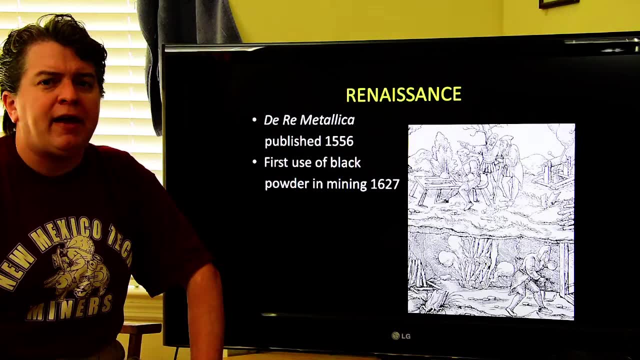 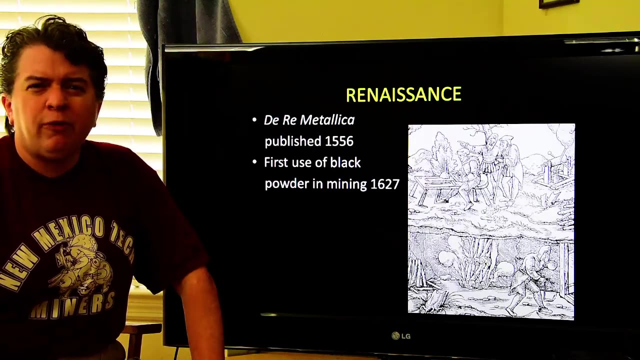 This is a reconstructed Roman water wheel Now, once we get to the Renaissance. so basically the Romans were kind of this high point of ancient world mining and following the fall of the Roman Empire not really all that much changed in the mining industry. 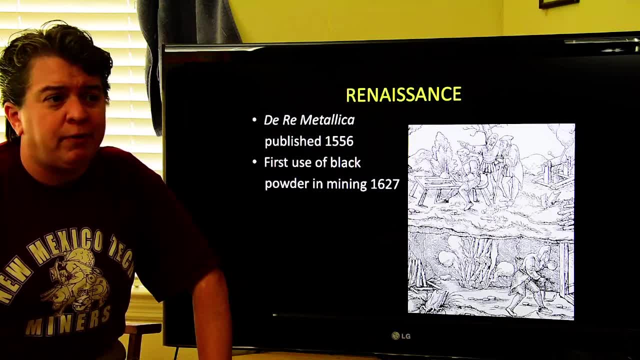 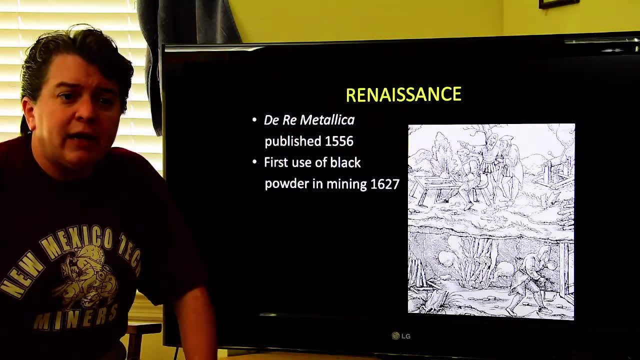 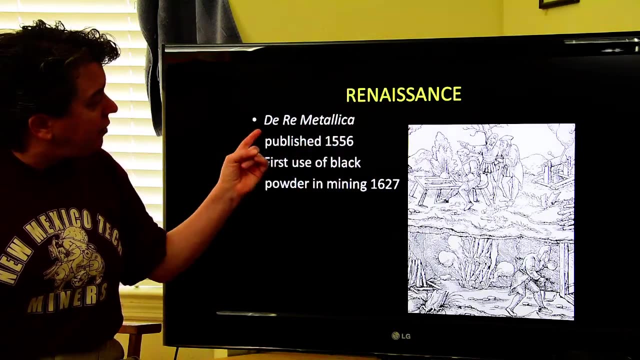 Really it just A Roman could have shown up in the Middle Ages and been like: yep, this looks pretty familiar. What really Changes come in the Middle Ages, And so we have Dei re Metallica or sorry. changes really come in the Renaissance. 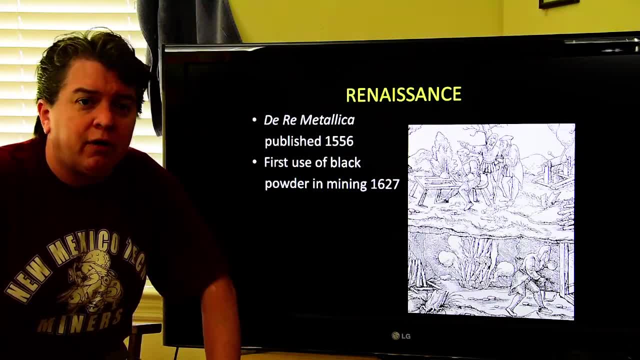 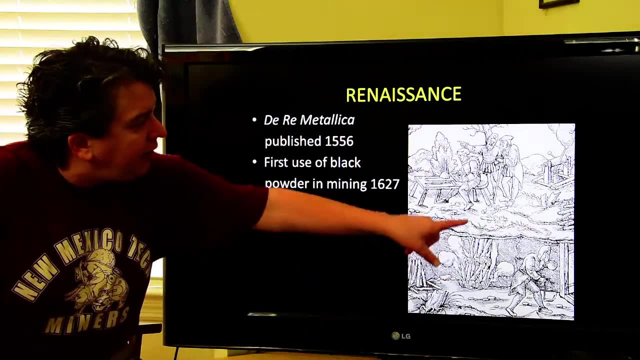 So Dei re, Metallica is a book. It's basically a textbook on mining that was published in 1556. that shows you all kinds of techniques. It's like fire setting. it shows how to build winches. it shows how to build smelters of. 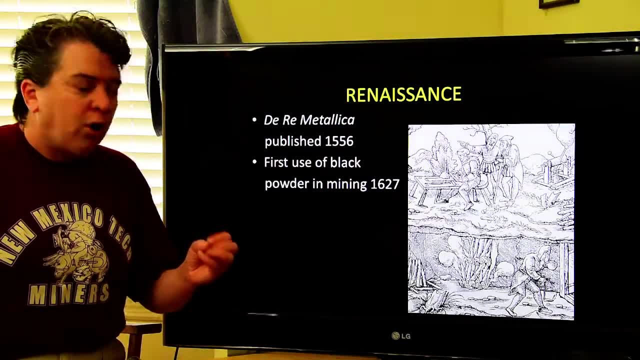 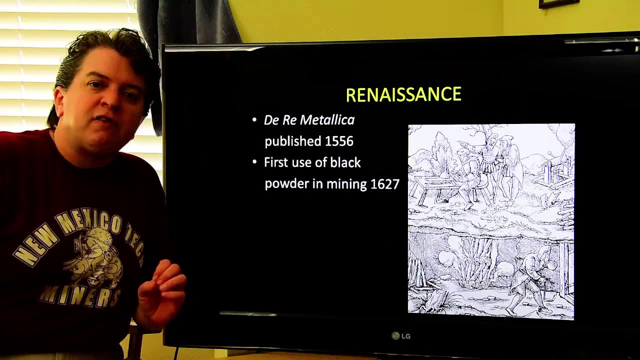 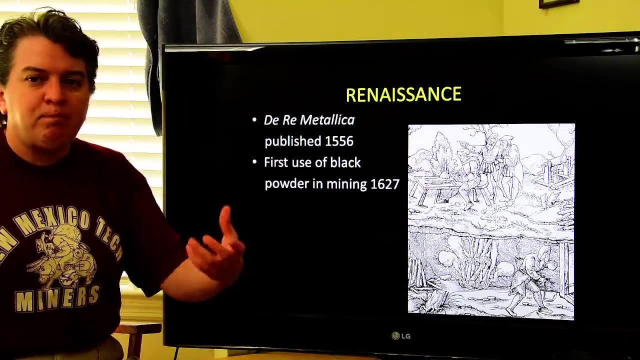 different kinds. So a really important book. And then there's also the first use of black powder in mining. the first use of explosives in mining is documented in 1627.. And that's really. our next big advantage is this use of explosives. 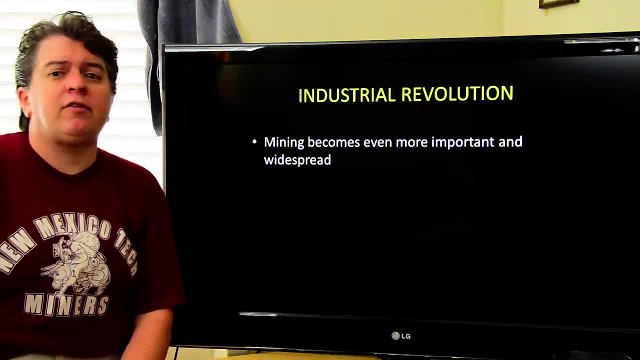 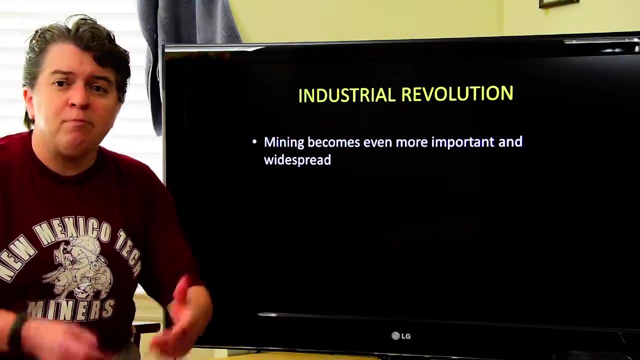 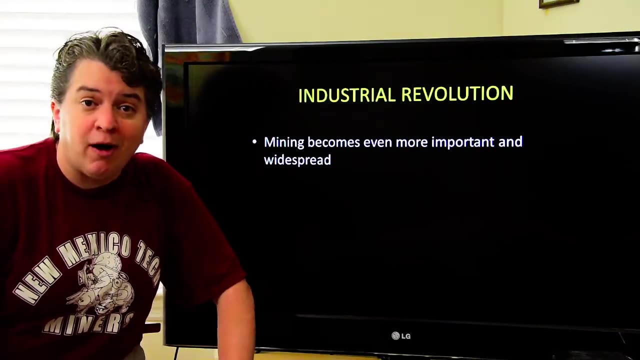 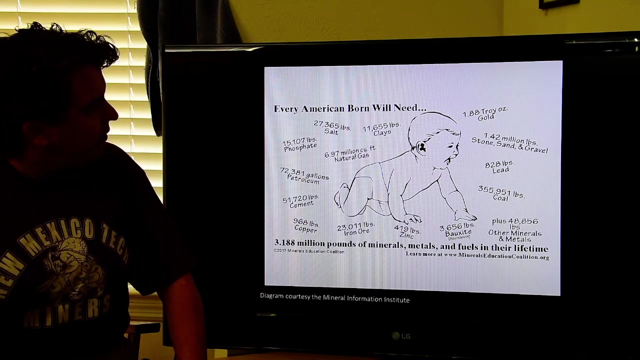 So that one. And then we leave the Renaissance and ultimately eventually get to the Industrial Revolution, where mining becomes even more important and widespread because it's making all of these amazing things that we have for our convenient modern day life. So this is from the Mineral Information Institute. 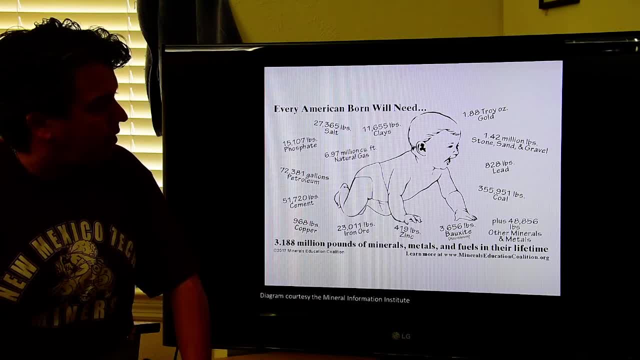 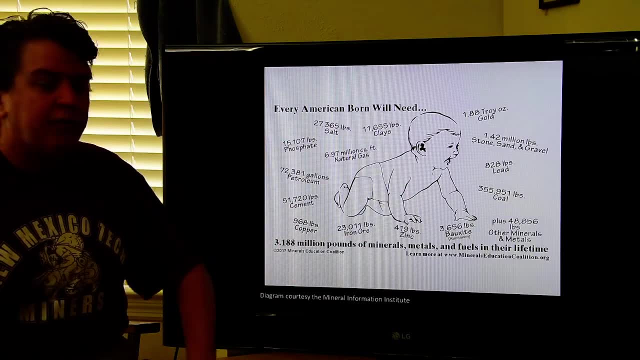 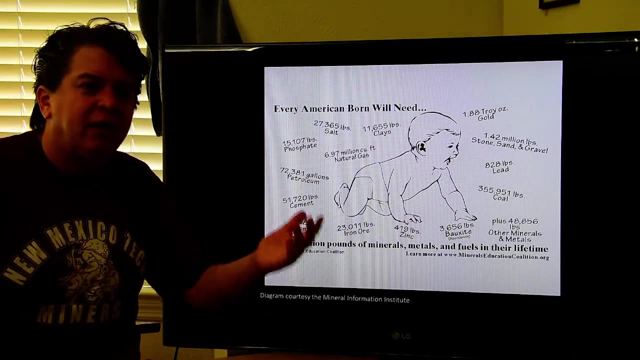 We call this the mining baby. This is every American born this year. Actually, this was 2017.. But close enough. It's going to need a certain amount of different materials And, of course, these are estimates. It's taking into account the average lifespan and the average number of cars people own. 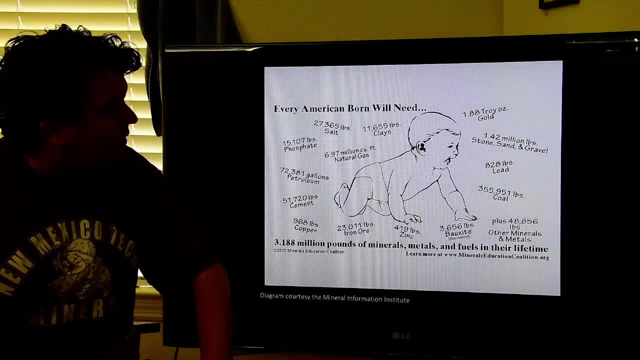 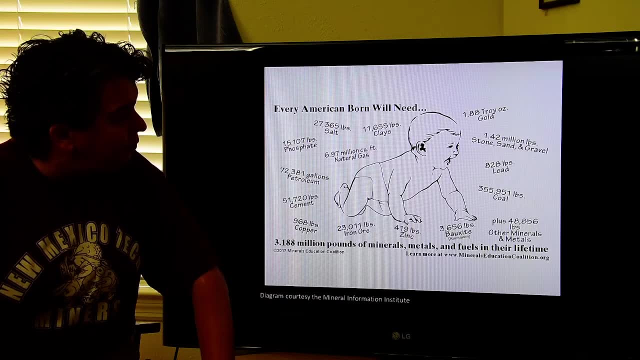 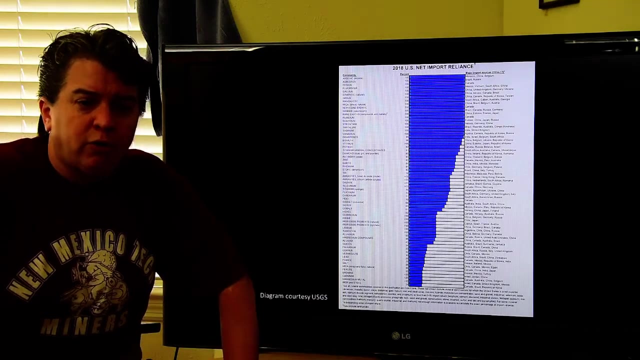 and all that kind of stuff. But it does give you a good idea of materials that you might not even realize that you are using. And then I always like to put this one in: This is the use of black powder. This is the US net import reliance for different minerals and commodities. 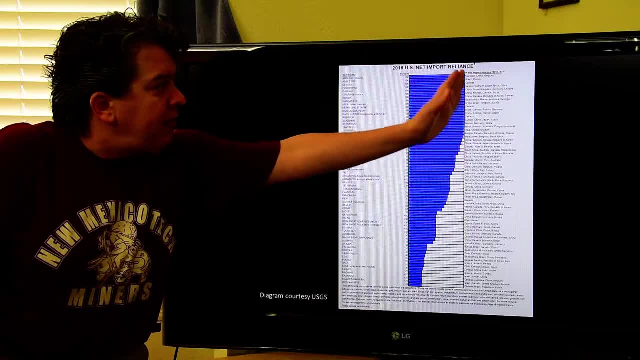 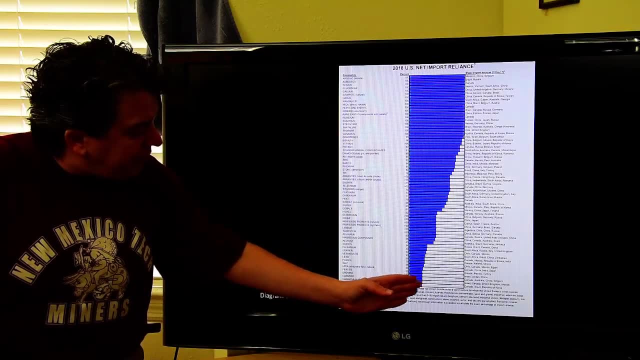 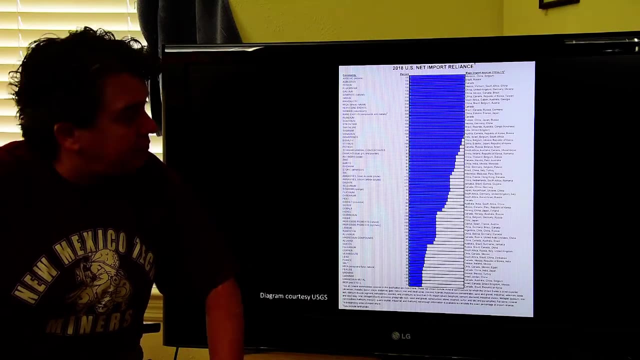 So basically, the farther to the right we are, that means that we're completely reliant on imports And the farther to the left the blue bar is, that means we actually don't use that many imports and use a lot more domestically produced stuff. 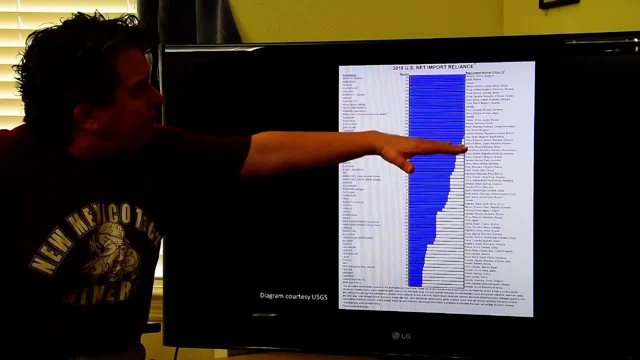 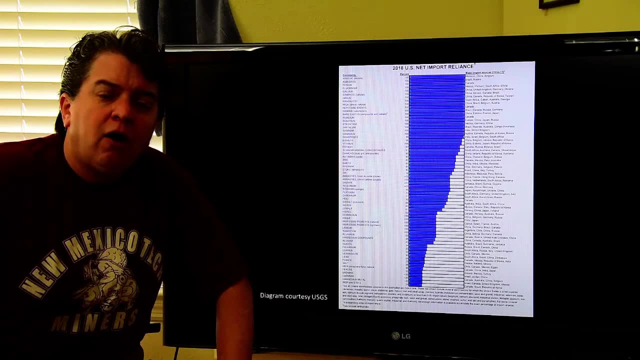 And so what? this is showing us all the way down to here, everything above this. we don't produce any of that in the United States and rely 100% on other countries for that commodity. And what other countries do we rely on? 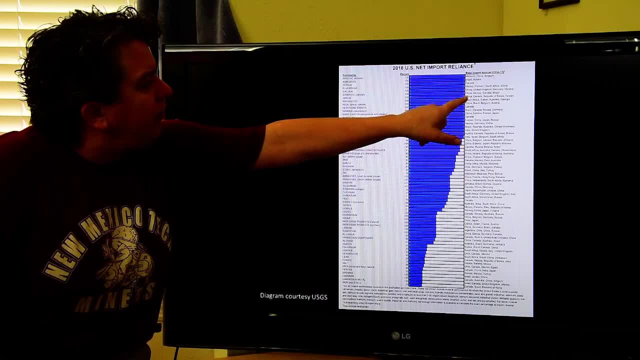 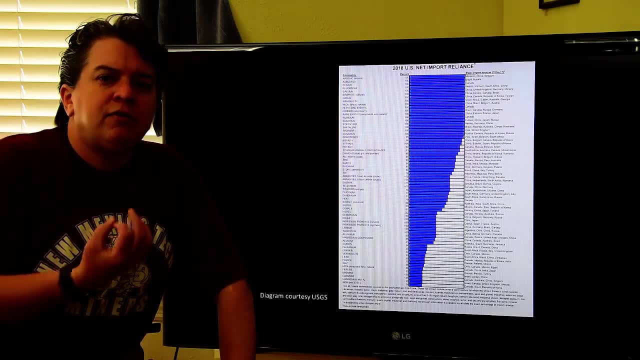 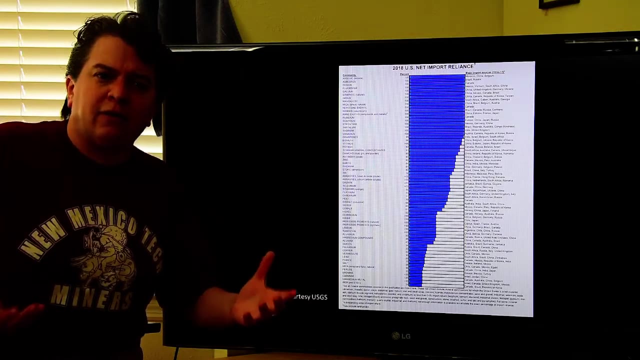 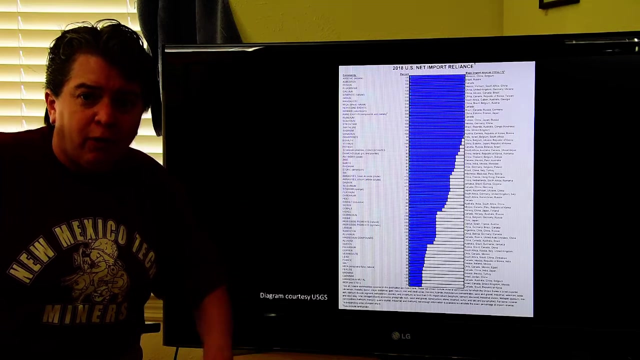 We see Morocco, Brazil, Canada, China, China, China, South Africa, China, Canada, China. You start seeing this and you need to think about minerals in the grand scheme of also the political climate. So oftentimes it's very easy to yell: let's have a trade war with China. 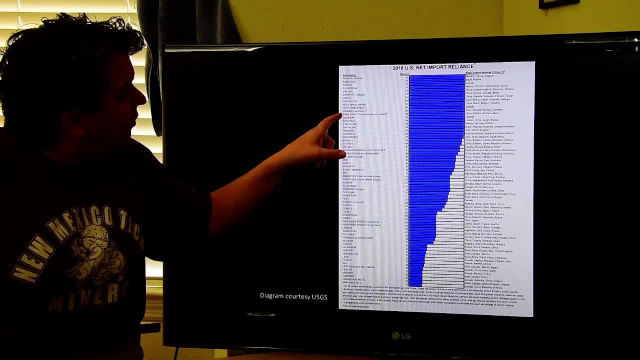 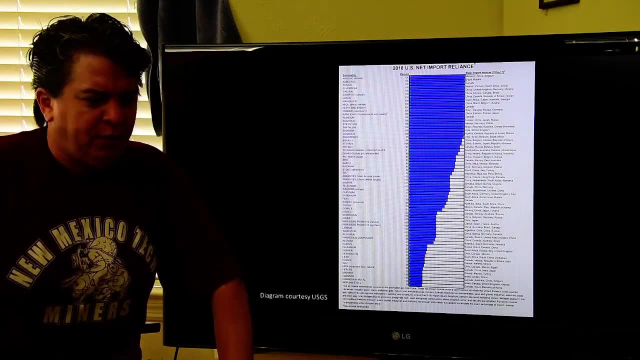 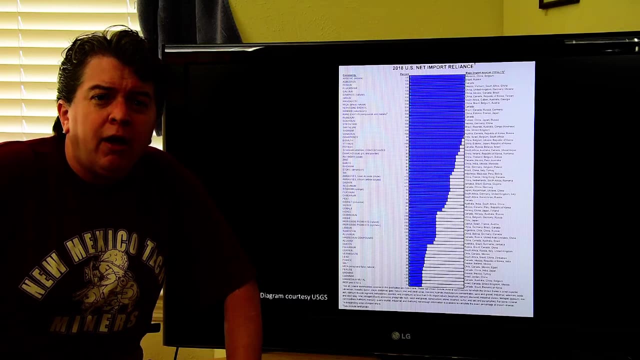 But then you start realizing that we rely on that country for things like, well, scandium and rare earth elements and things like that. And you might say, I don't care about scandium or rare earth elements, But considering that you're probably watching this on a computer or smartphone and the transmitters 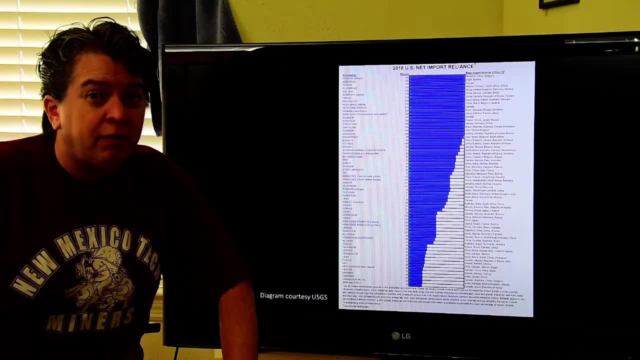 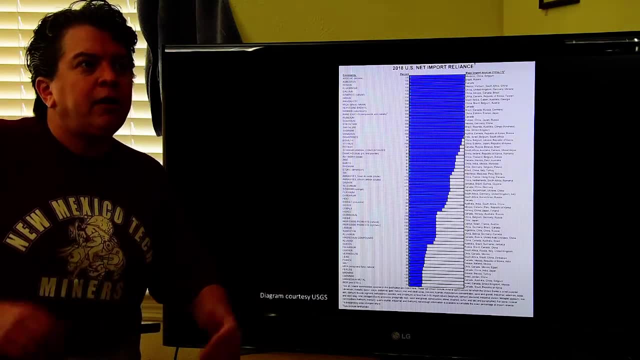 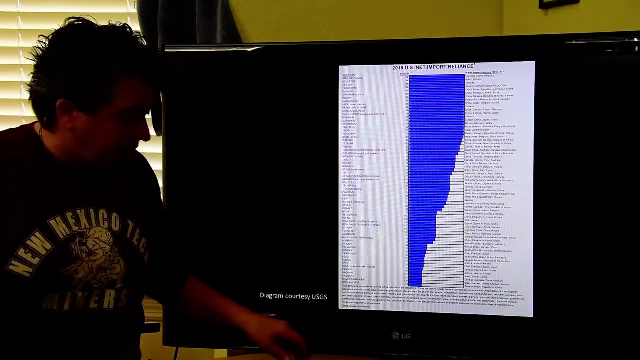 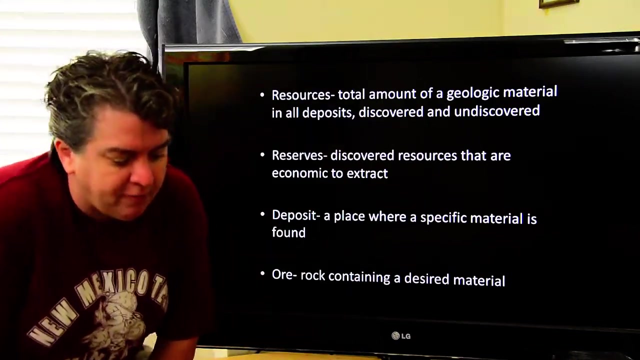 work without those. you probably do care about those rare earth elements and some of these other weird things there. So just realize that the mining industry is vital to our modern day lives and it can actually be kind of it can be complex. All right, so some vocabulary that you're going to have to know for this topic. 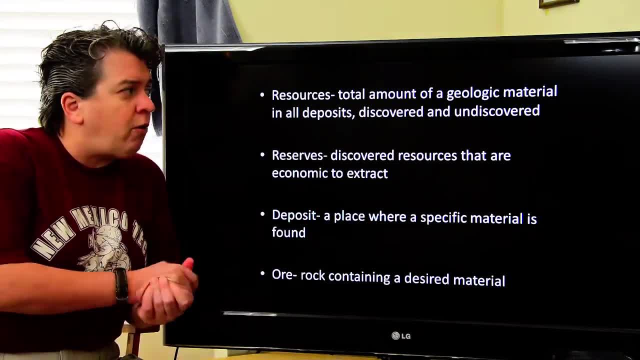 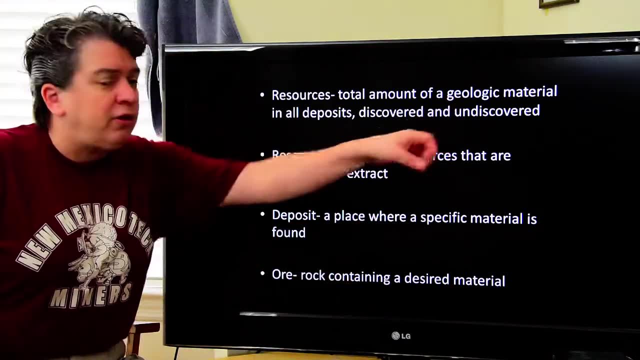 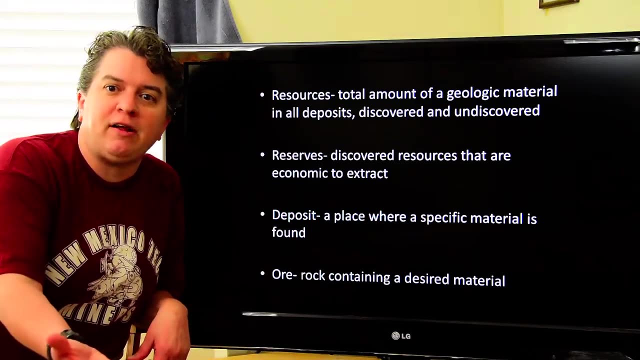 Resources, Resources, Resources are the total amount of a geologic material in all deposits discovered and undiscovered. So when we're talking geologic material, that's whatever the important thing we're looking for. So it could be like copper resources or iron resources or it's whatever that commodity. 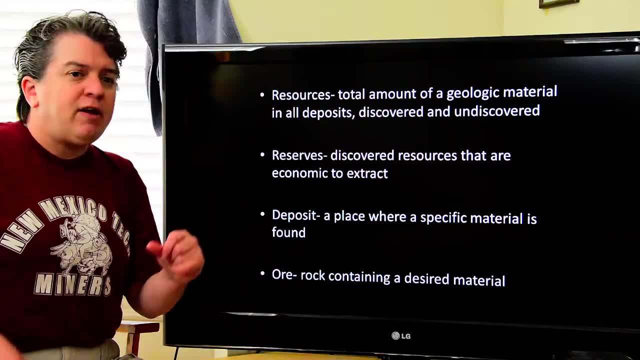 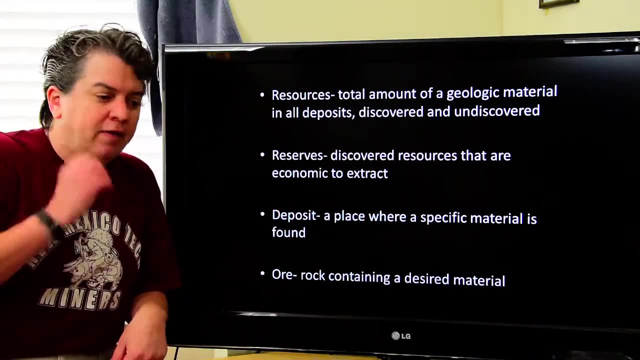 that we're seeking, That's this geologic material And resources are all of that in the entire world, Whether we know about them Or whether we don't know about them. And you might say, well, how do we not know about them? 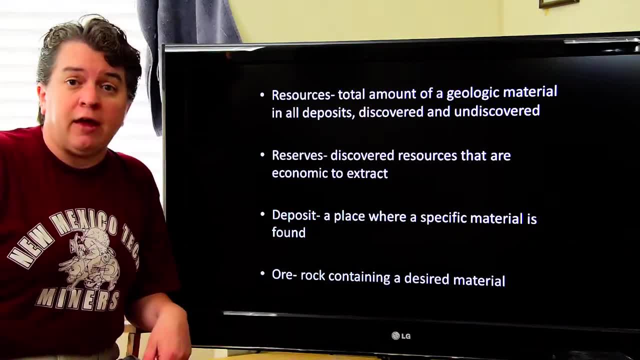 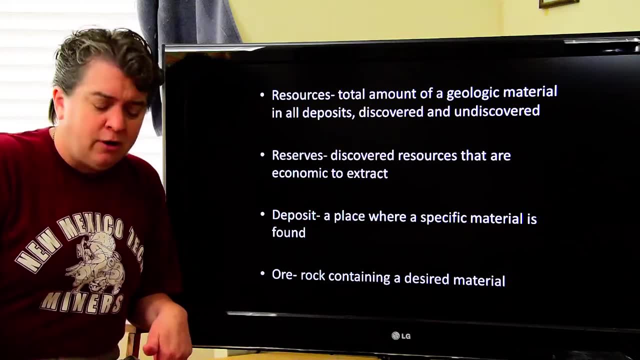 You know, people have been exploring the world a lot, and yes, they have. But think about things like Greenland. There's a whole lot of ice covering Greenland. Do we know what's under all of that ice? Not necessarily. What about all the oceans? 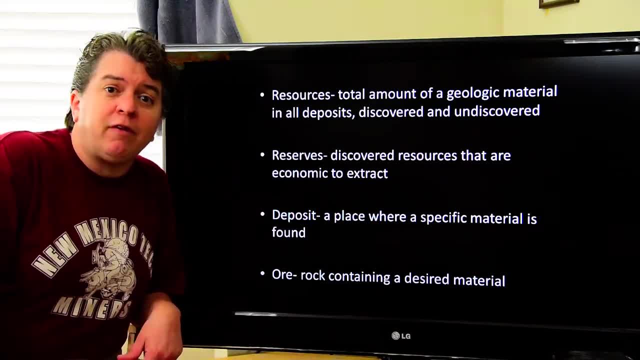 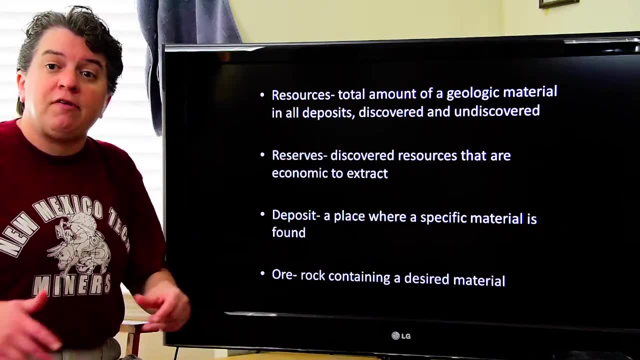 Do we know exactly. Maybe there's a copper deposit sitting on the ocean floor and we just don't know about it. That would count in the undiscovered resources, These things that exist but we don't know about them yet. And then, of course, there's discovered ones. 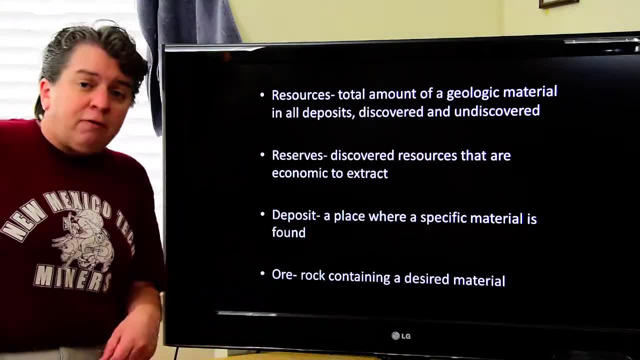 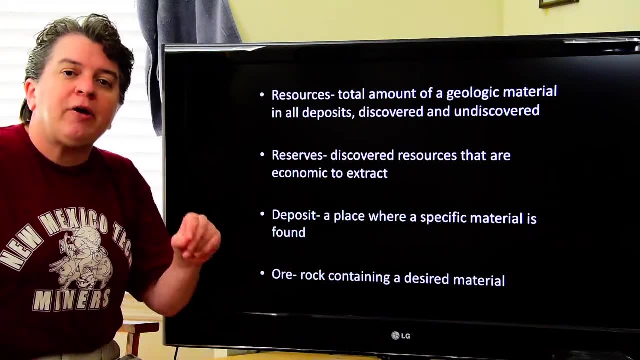 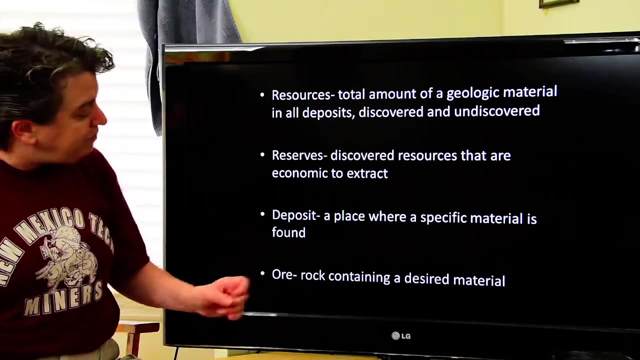 Ones we know about Now. resources are different from reserves. Reserves are discovered resources that are economic to extract And- that's a very important thing. We can actually make money getting this stuff out of the ground Now. a deposit is a place where this specific geologic material is found. 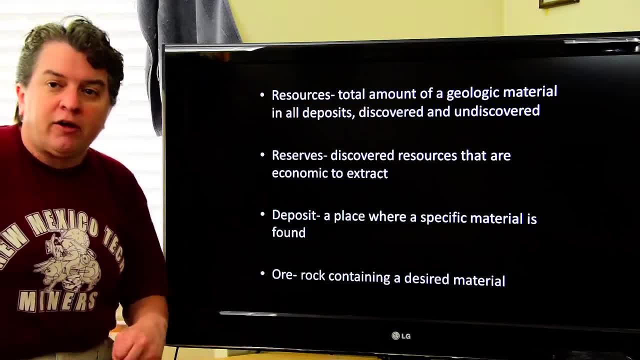 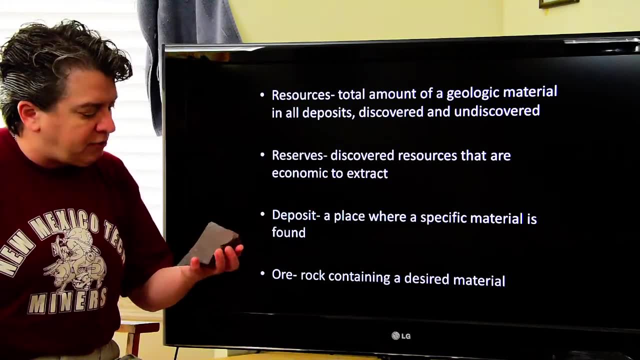 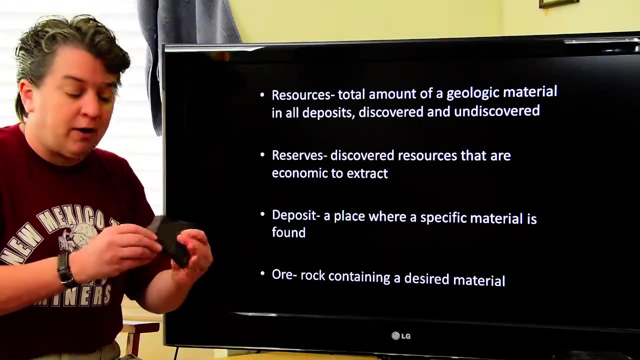 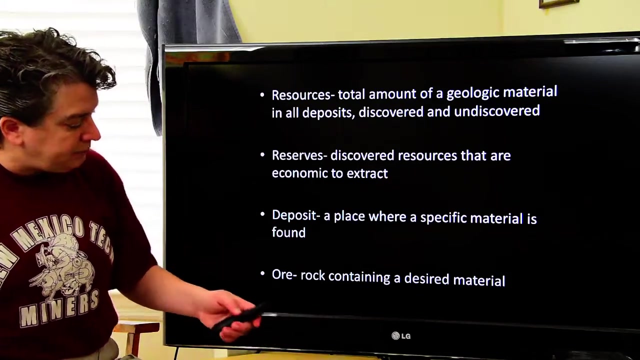 And ore is rock containing the desired material. So, for example, this happens to be a piece of iron ore that I just have sitting near my TV, But it's an actual rock that contains high enough amounts of iron that we could process this and make money doing that. 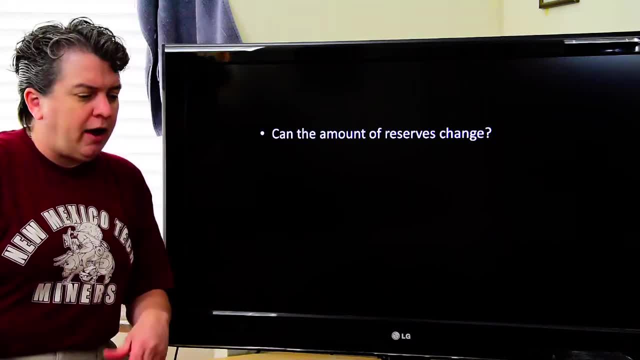 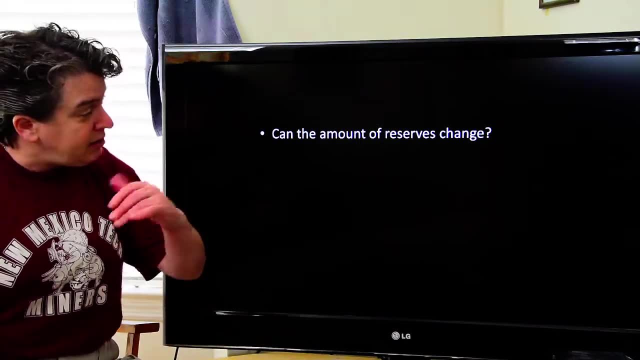 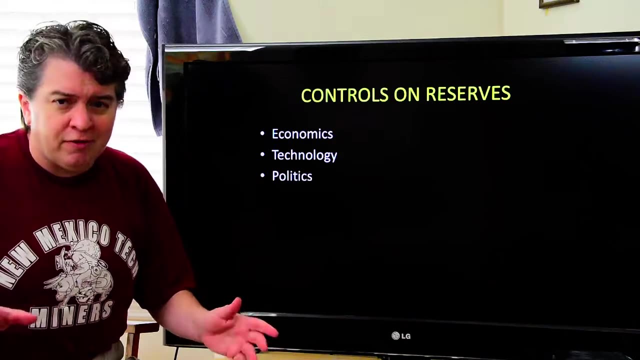 Now, can the amount of reserves change? And I hope all of you guys are sitting there at home or wherever you're watching this and you're like, yeah, of course reserves can change And yes, they can And things that affect reserves. There's hundreds of them, but ultimately you can kind of boil it down into three main groups. 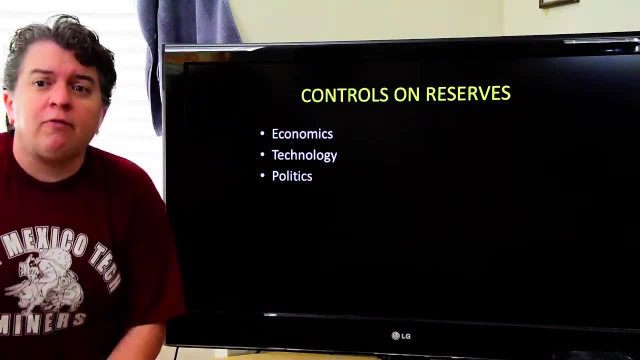 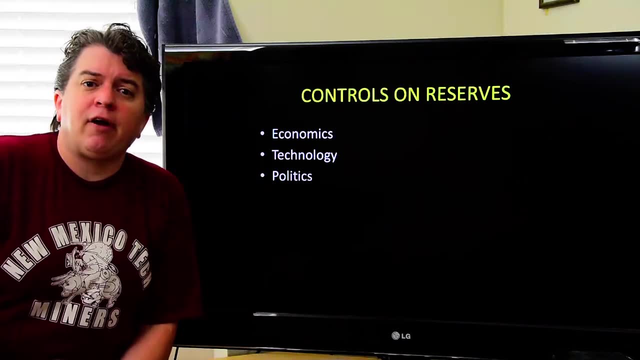 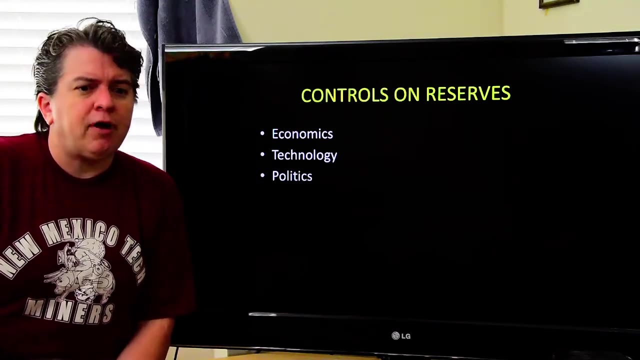 The economics of the time can affect the amount of reserves you have. Economics would be things like supply and demand, The price of a commodity. For example, when I taught at Michigan Tech, the price for a pound of copper was something like 70 cents. 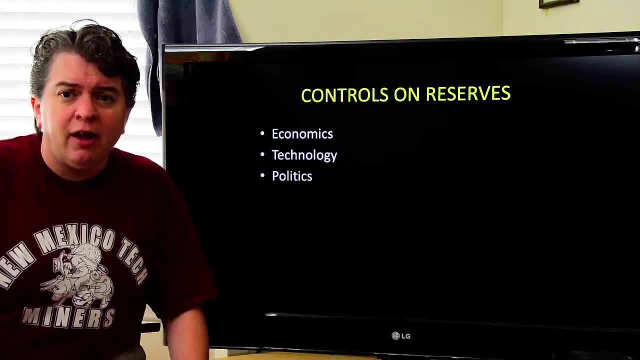 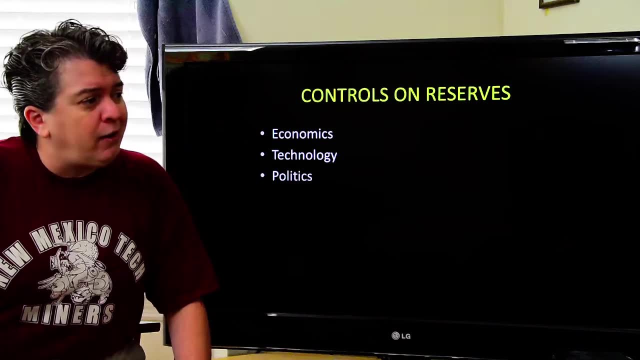 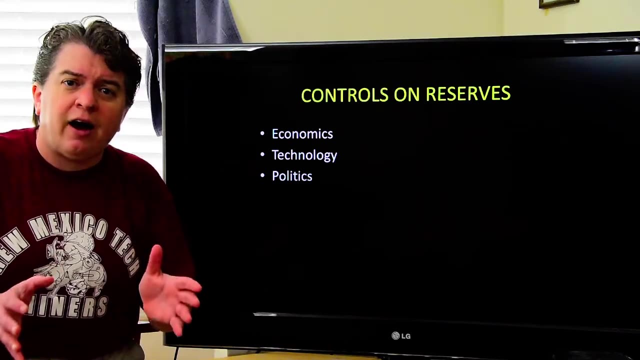 So you could have a pound of pure copper and you'd get 70 cents for it. Today it's closer to around $2.40.. So think about that. $2.40 is a significantly higher amount than 70 cents, Right. 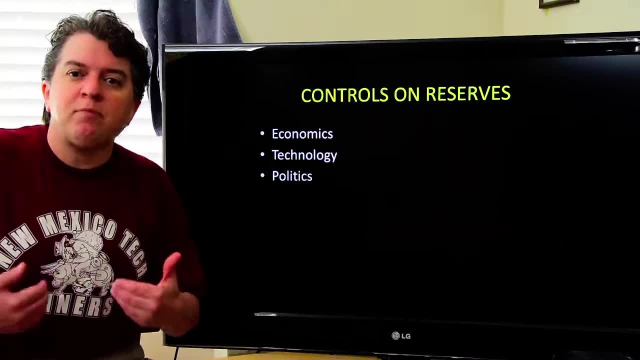 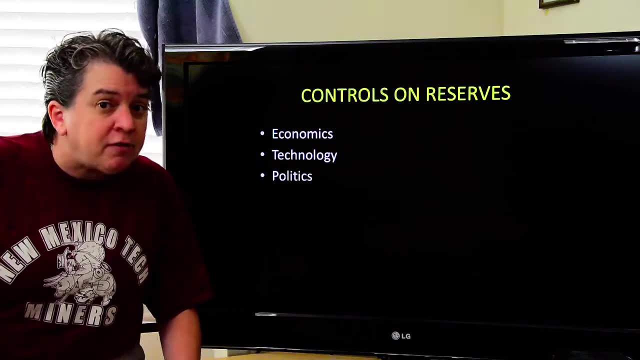 So there used to be deposits that you could not make money on selling at 70 cents a pound, but you could make money on selling for $2.40 a pound. So the economics of the time, the demand for a material, the supply in the market, that 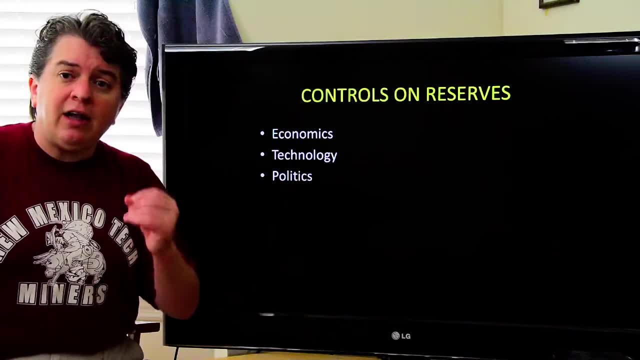 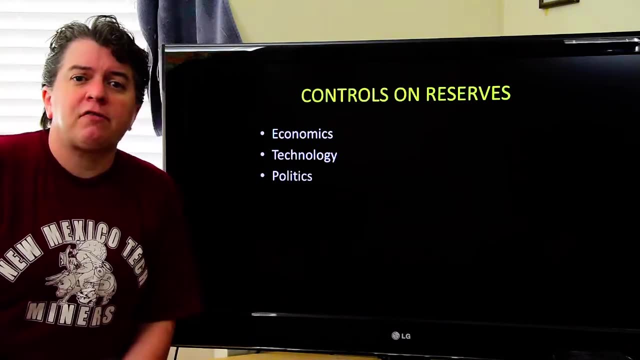 can affect the amount of reserves we have. Technology can also affect this. You know, if we develop a newer technology that makes it cheaper to extract things, you're going to have more resources, things out of the ground- well, that might. that might make some resources now. 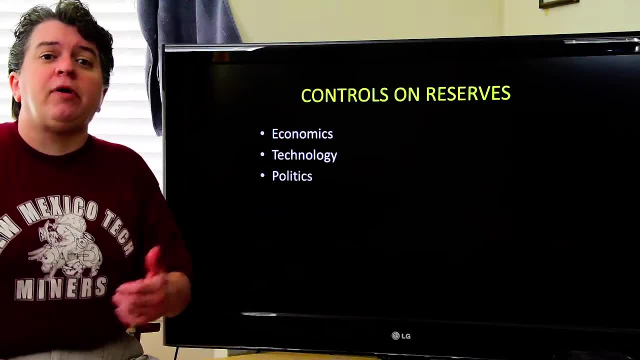 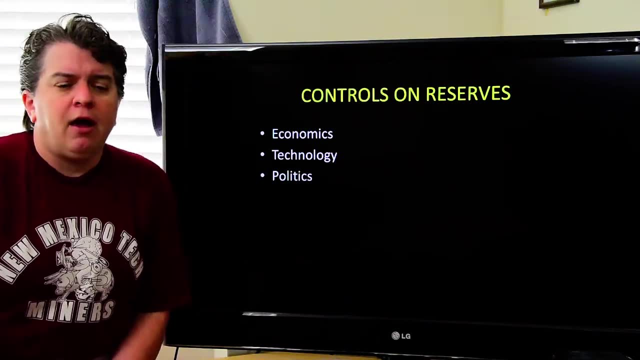 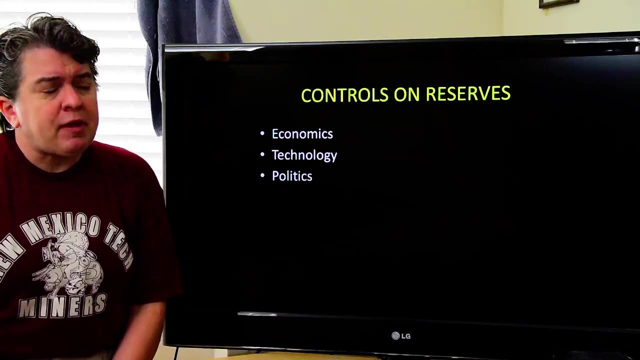 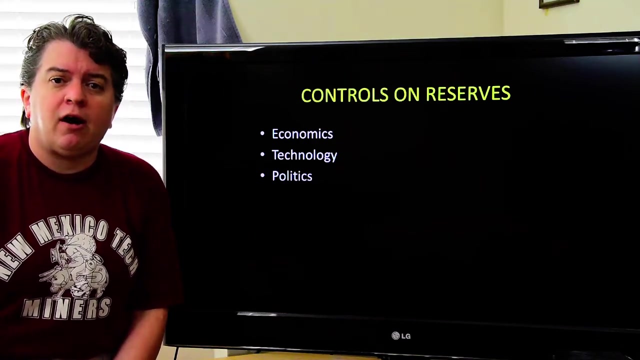 become economic. and then there's always the political situation, and this is comes in two, two very different ways. for example, there's always the legalities of things. within Wisconsin, up until last year, extracting metals was illegal. you, you could not mine for metals in that state because there was a law against it. 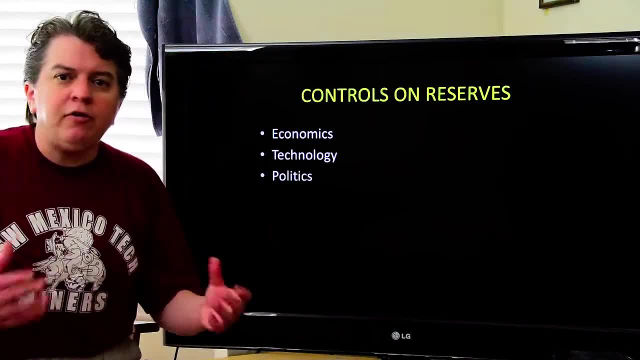 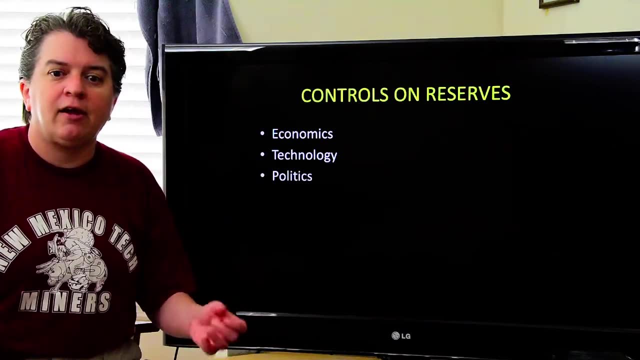 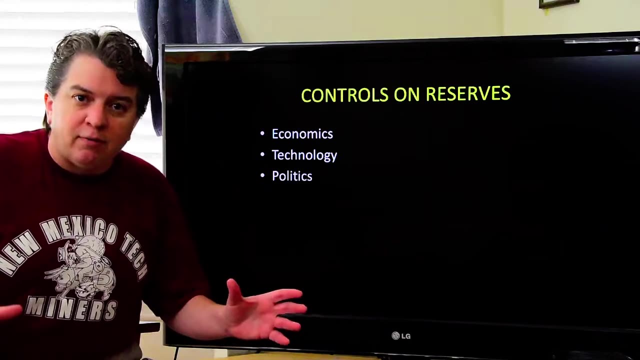 and even though they have a huge copper deposit in the northern part of the state, that if that was out in New Mexico or Montana or something, people would be extracting it because there was a law in place, people couldn't touch it. so doesn't matter how rich that deposit was, it's still a resource. 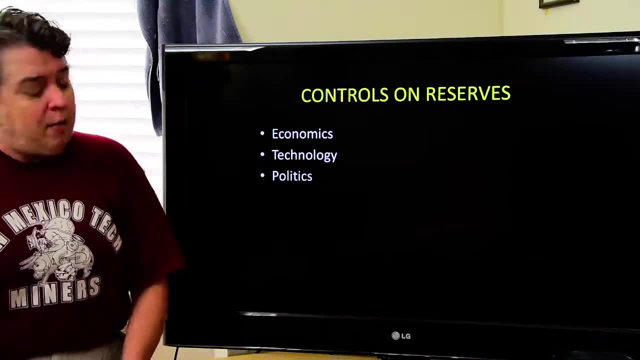 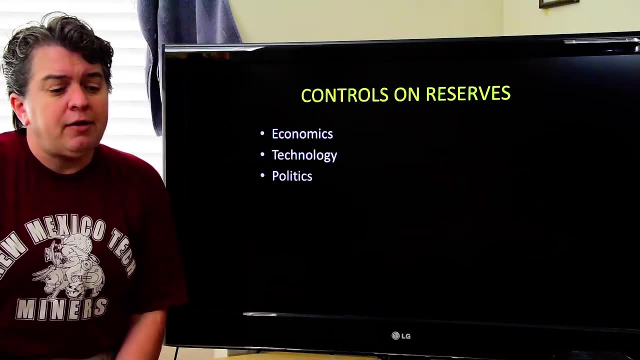 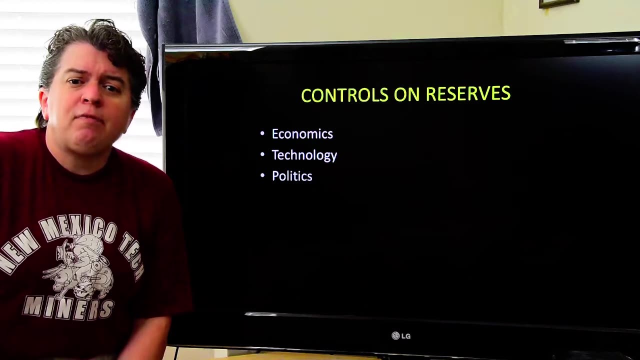 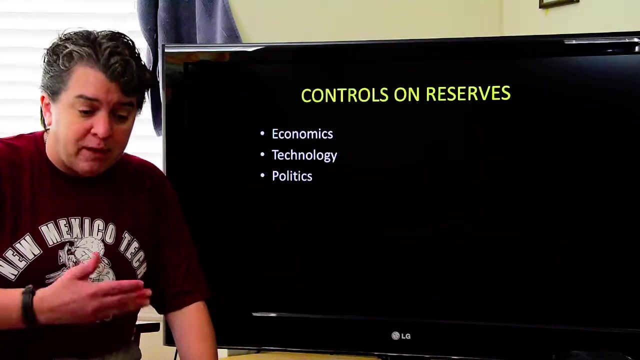 because it was off-limits legally. but politics also get involved when it comes to the stability of countries. you know, you places like parts of Central Africa or Afghanistan. these places actually have some very, very rich mineral deposits that, if they were located in other places, people would be. 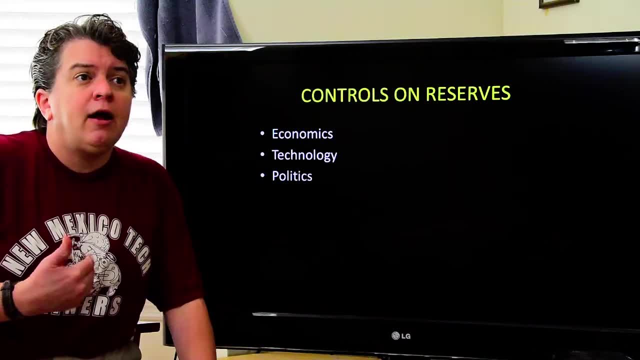 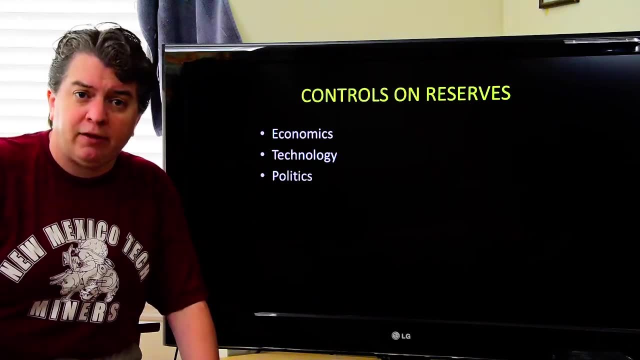 exposed to and they would not be able to access them and they would not be able to extract it. however, companies are very hesitant to invest in some of those places because of the political instability right. they don't know how safe things are going to be for their workers. they don't know how, how, if the 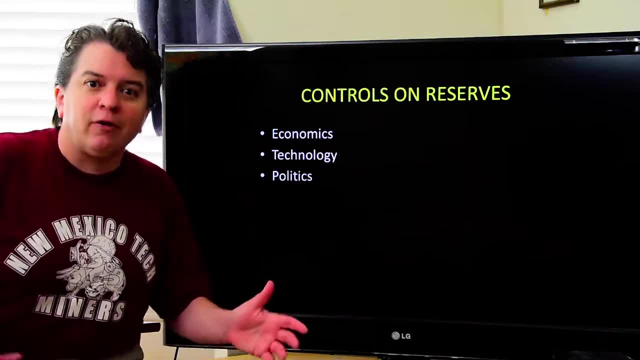 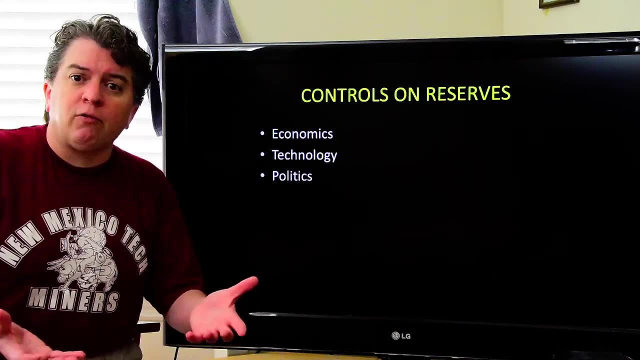 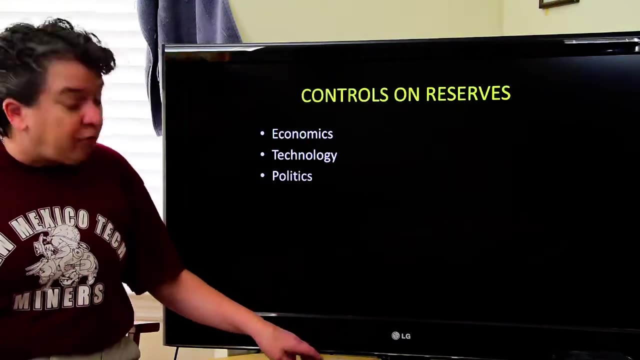 government's going to still exist tomorrow or if there's going to be some kind of weird rebellion or revolution, and so sometimes, even if there are rich mineral deposits in places, during that time people tend to look very 모�. ANNOUNCER. basic mixture: people stay away. 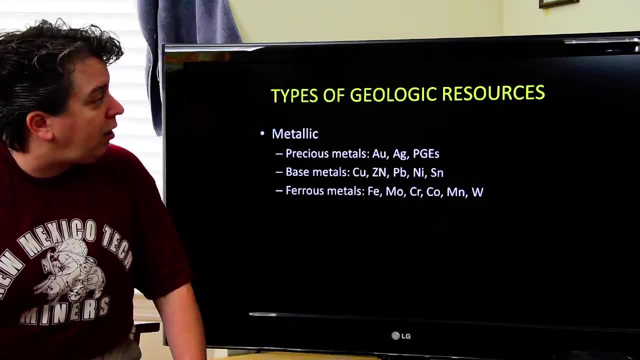 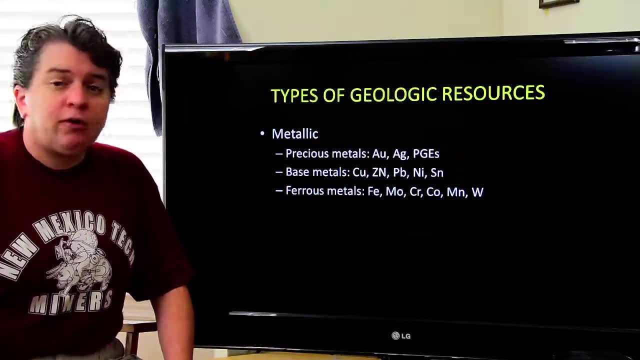 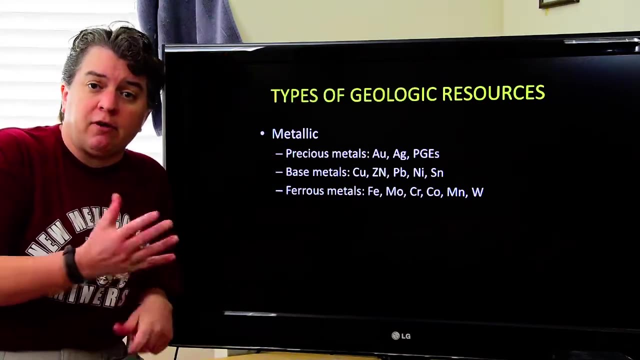 from there, simply because of the political instability of the region. so, anyway, those are some of the things that control our reserves. now. there are different kinds of geologic resources that we extract and use. we have our metallic resources. these are going to be metals that are extracted, and that's. 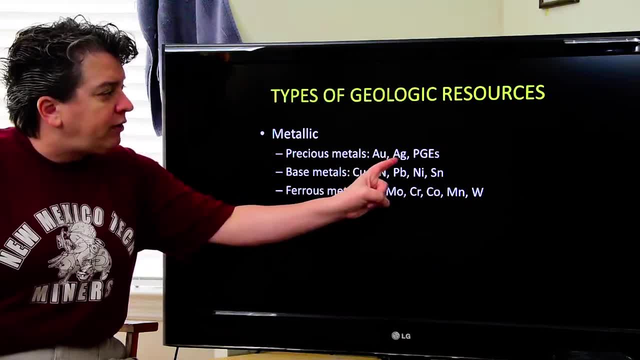 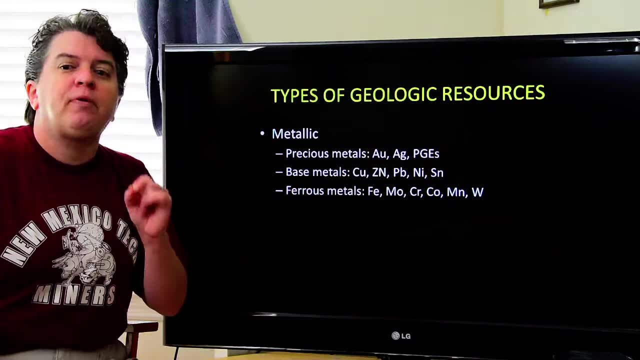 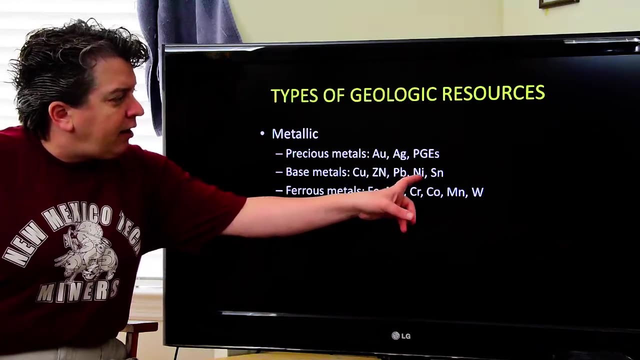 broken down into three different groups. we have the precious metals, that are, which are gold, silver and PGEs- PGE stands for platinum group elements. We also have the base metals, which are things like copper, zinc, lead, nickel and tin, And then we have the ferrous.